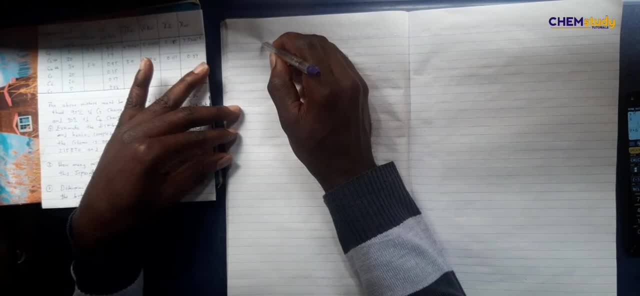 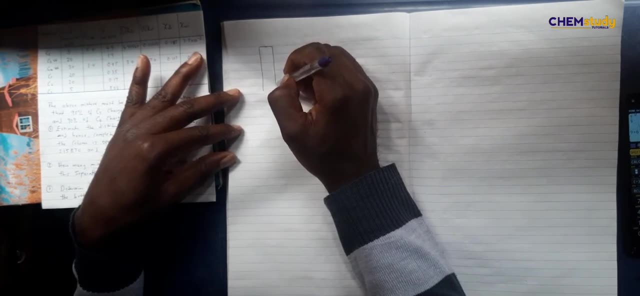 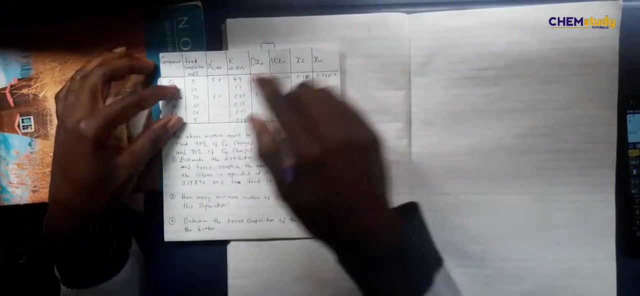 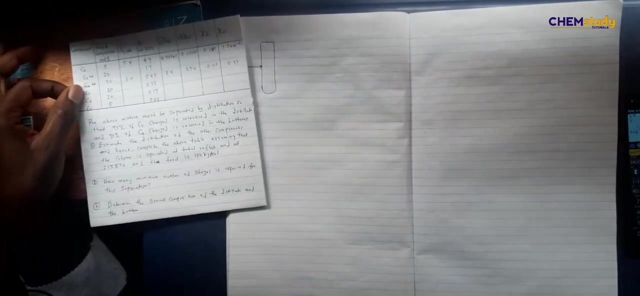 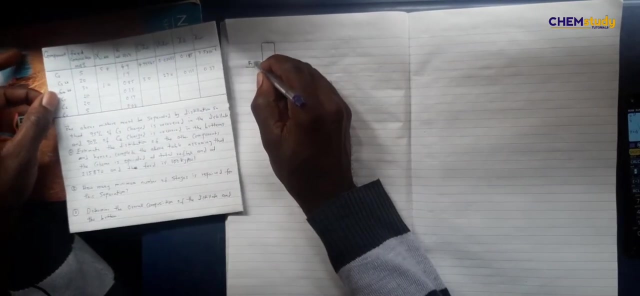 a distillation column that way to help visualize the problem, making it easier to tackle. so we have a feed now all of these components are going into the feed. okay, these are charged into the system. that's the feed over here. and remember, the question said the feed is 100 kilomoles. kilogram moves, so 100 kilogram mode. now what comes out at the bottom? 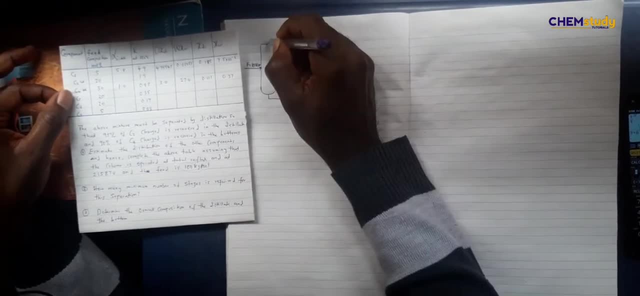 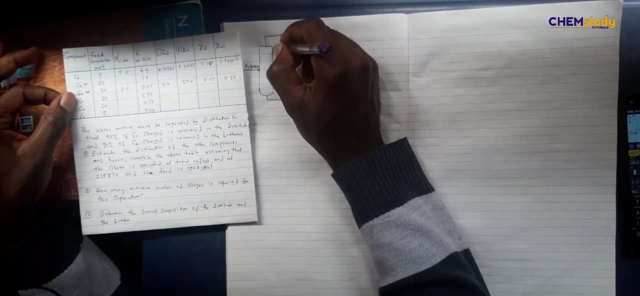 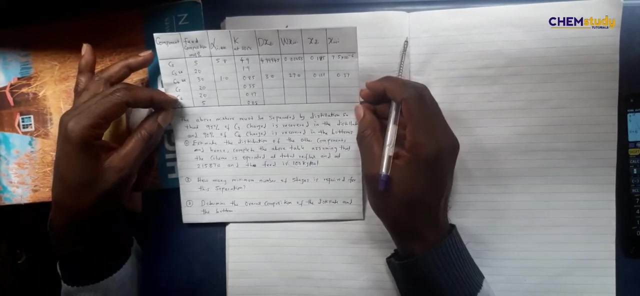 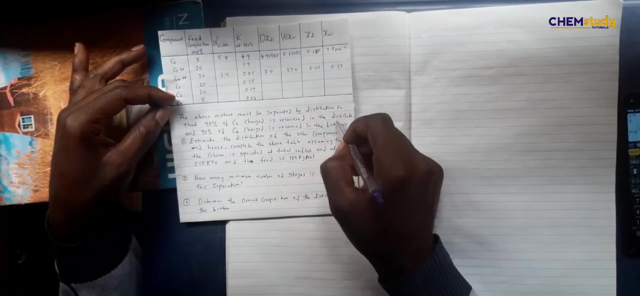 is the w, then we have the, have a condenser. here, we have the reflux and the distillate d. okay, now the above mixture must be separated by distillation, so that 95% of C3 charge is recovered in the distillate and 90% of C4 charged is recovered in the bottoms. 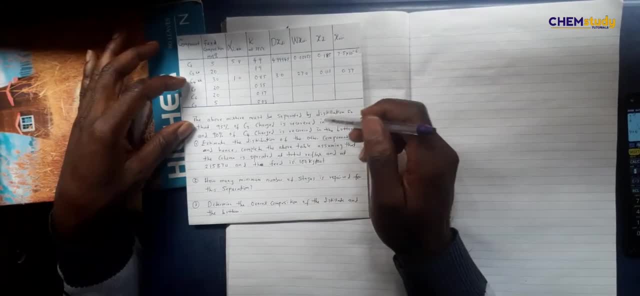 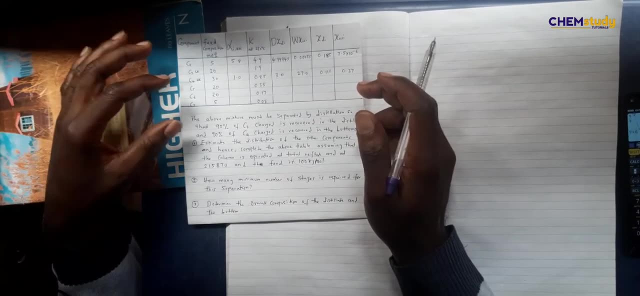 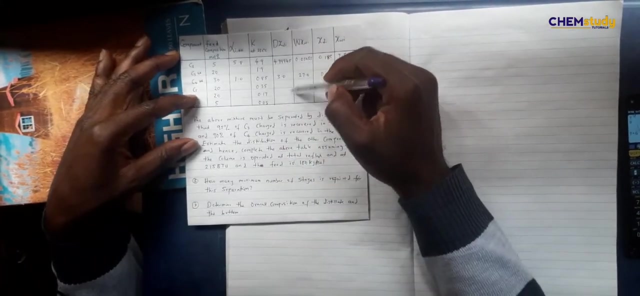 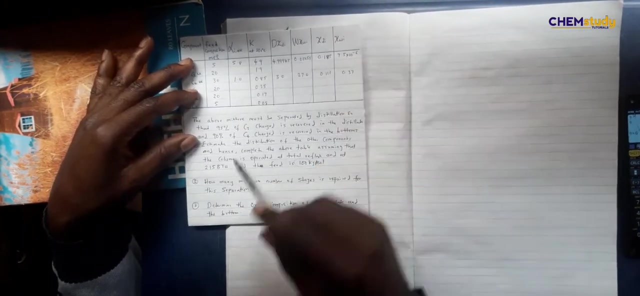 so question one estimates the distribution of the other components and hence completes the above table, assuming that the column is operated at total reflux. so what this question one is saying is that we should estimate the distribution, that's this column and this column. so what we would be doing would be how to fill this column and this column. then question two says how many. 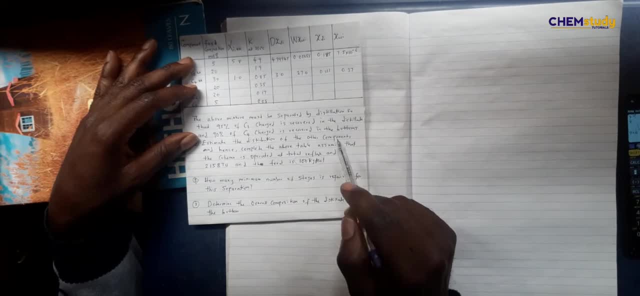 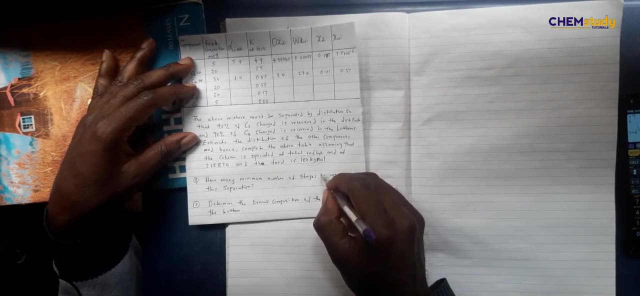 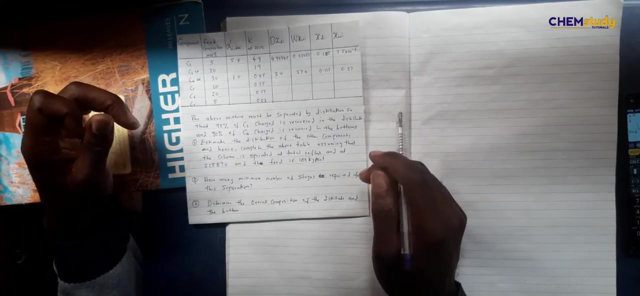 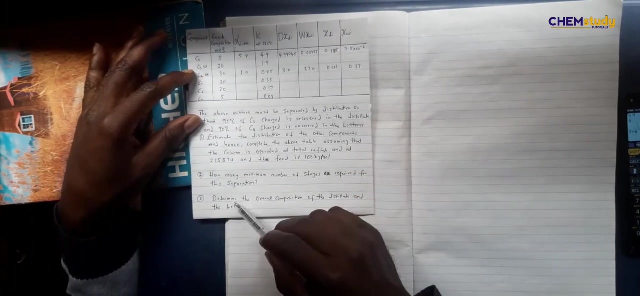 minimum number of stages is required. how many minimum number of stages should be required are required for this separation? so we look for the minimum number of stages, which is n, m would use fenske equation for that. then the last says we should determine the overall composition. 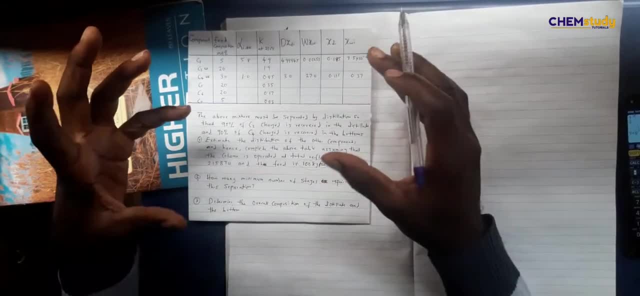 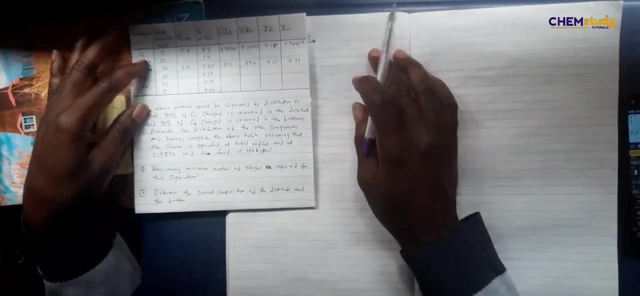 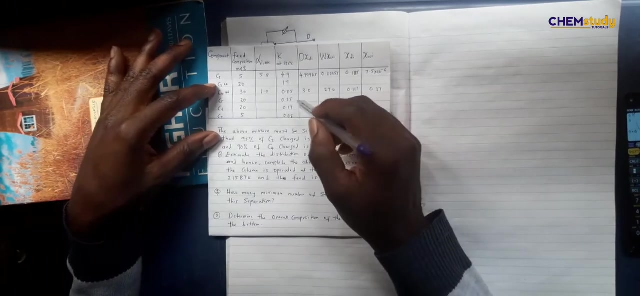 which is this and this, so we would solve all of them together. okay, one to three would solve all of them together. so how do we proceed? um, first, let me fill this column, because i think it would be very easy to feel, since we've identified our heavy, key component in the column, which is the end. that is the end of the column. so 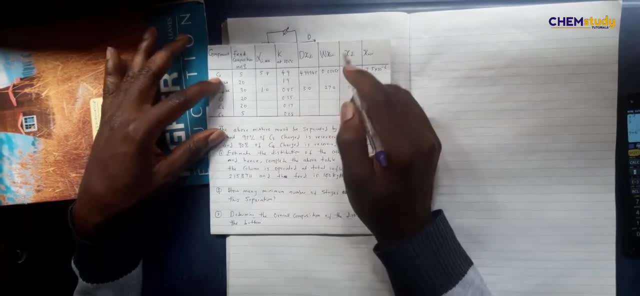 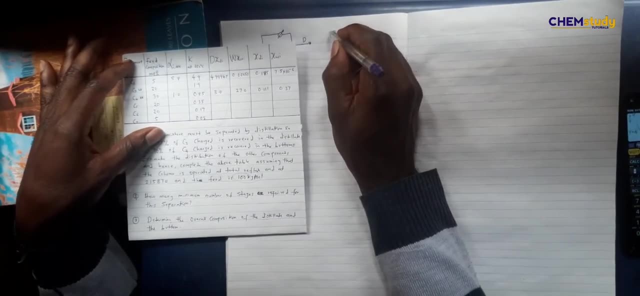 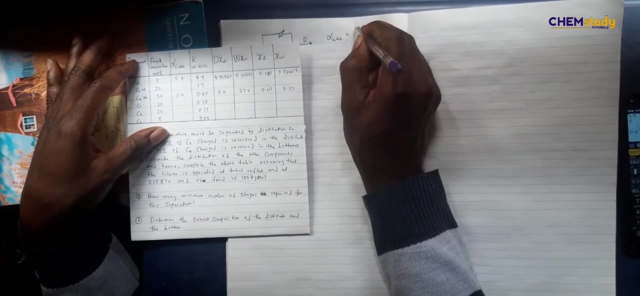 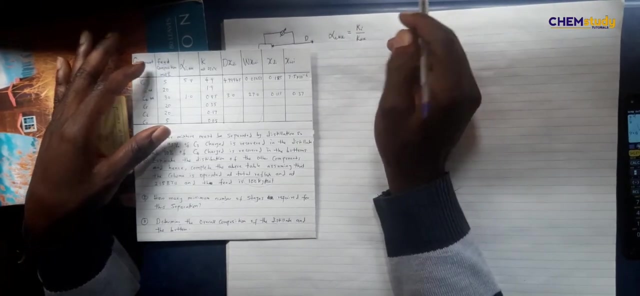 component as c4 and our light key component as c3- and let me just fill this column first before we begin anything. and we know that relative volatility of a component with respect to the heavy key is the k value of that component over the k value of the heavy key. so this: 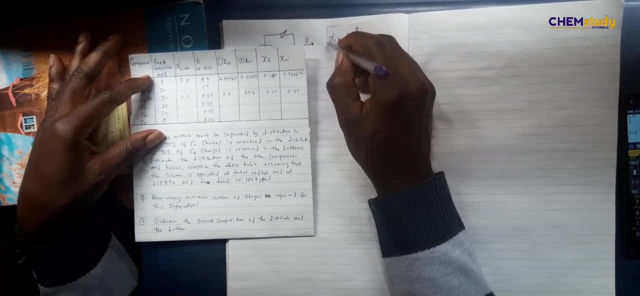 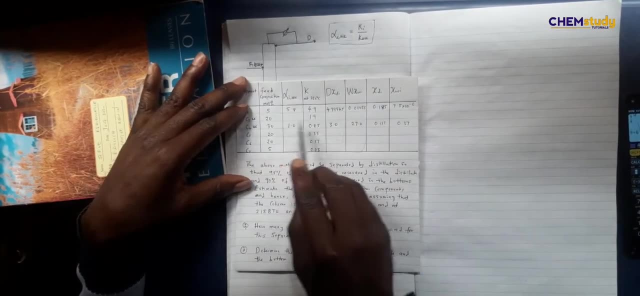 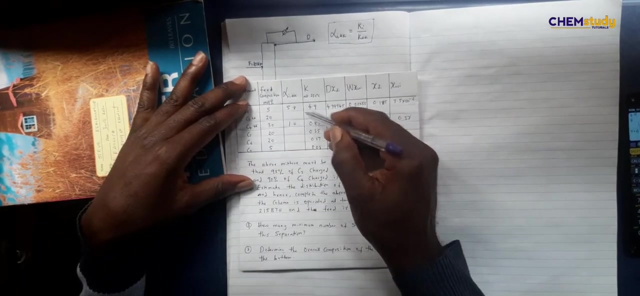 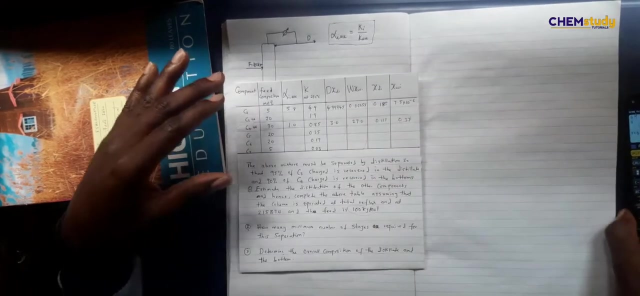 has been established in the lecture notes. okay, so to fill this table would simply be k- this is the heavy key. c4 to simply be 4.9 divided by 0.85, you get 5.8. then that's ki or khk down. you divide 1.9 divided by 0.85. 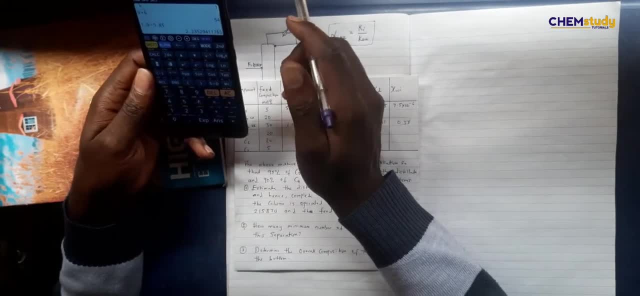 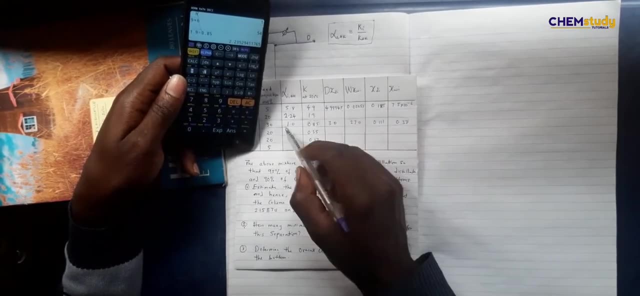 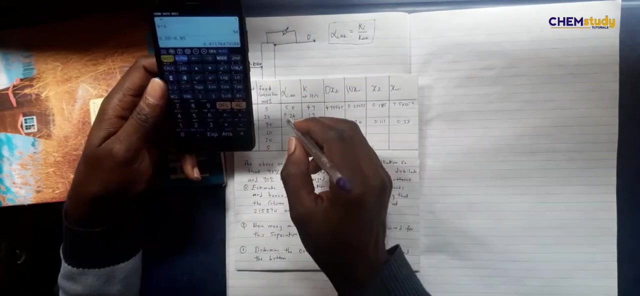 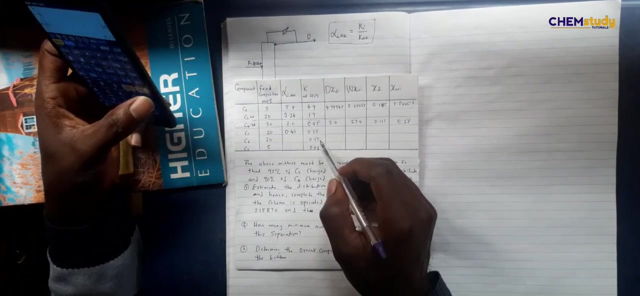 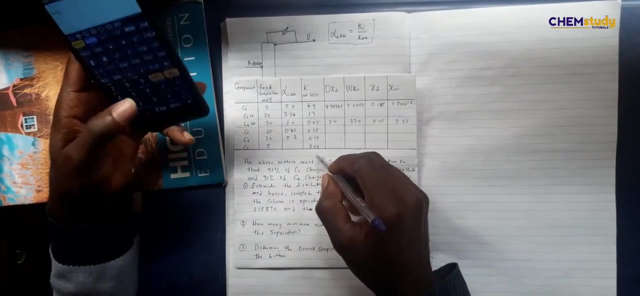 1.9 divided by 0.85, then 2.24. 0.85 divided by 0.85 is 1: 0.35 divided by 0.85, that's 0.41. now 0.17 divided by 0.85, that's 0.2, then we have 0.08. 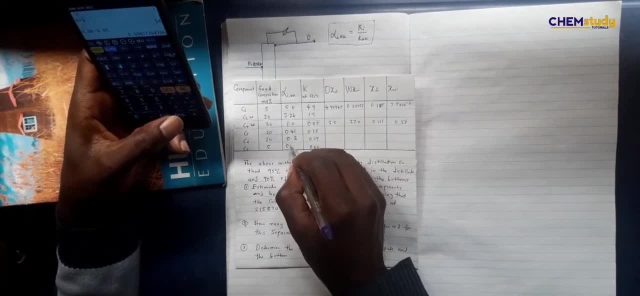 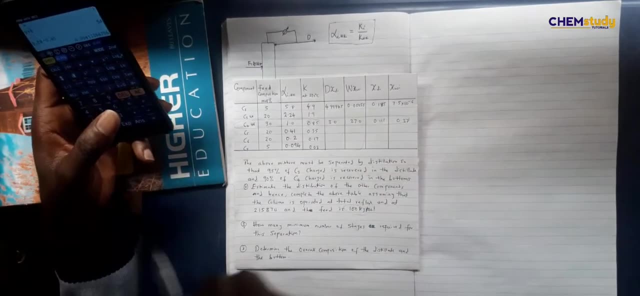 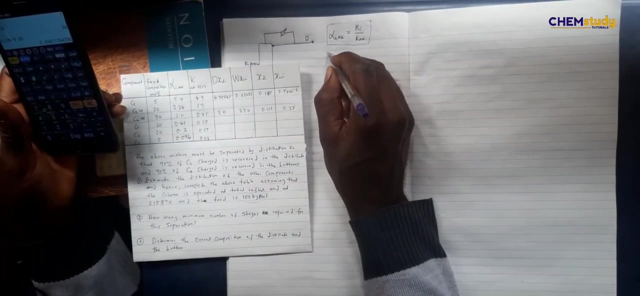 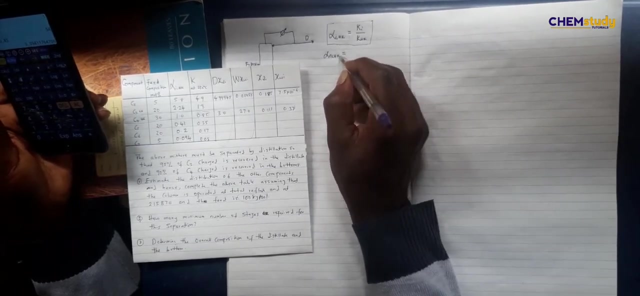 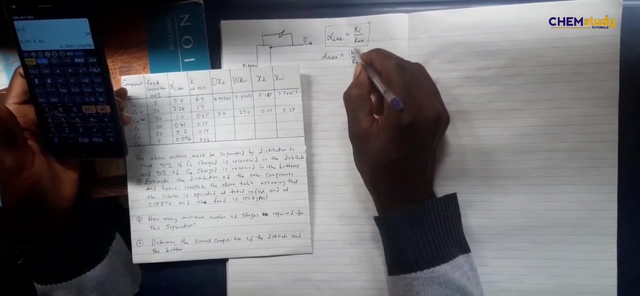 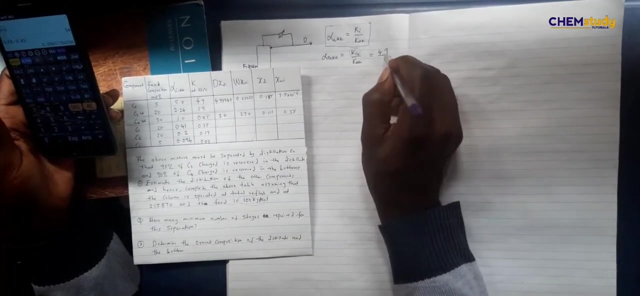 divided by 0.85, now 0.094. so this what we have. so it's very easy to fill this. remember to write it out. so that's alpha c2 h k is equal to kc2 over k h k, where kc2 is 4.9. 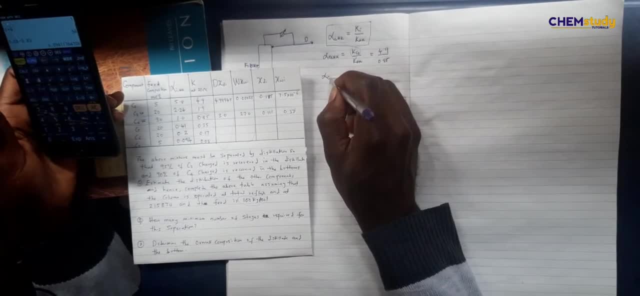 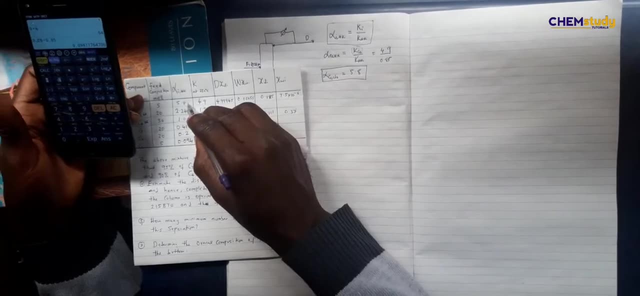 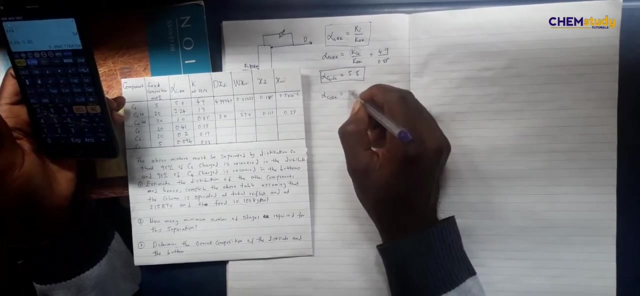 that's 4.9 over 0.85. so alpha c2 h chi becomes 5.8. that's how you got the first one. then the second one, alpha c3 hk is 1.9 by 0 point. that's 1.9 over 0.85. 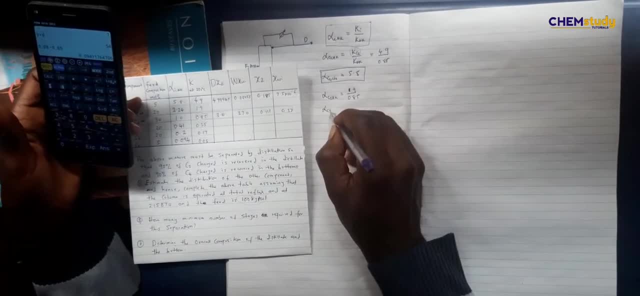 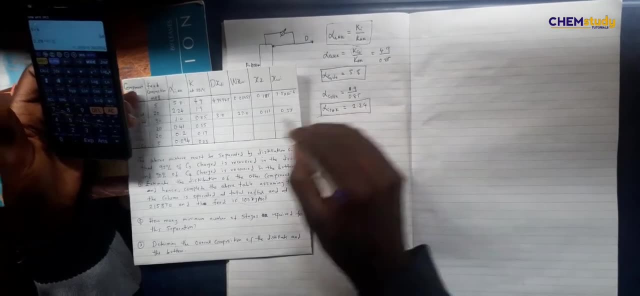 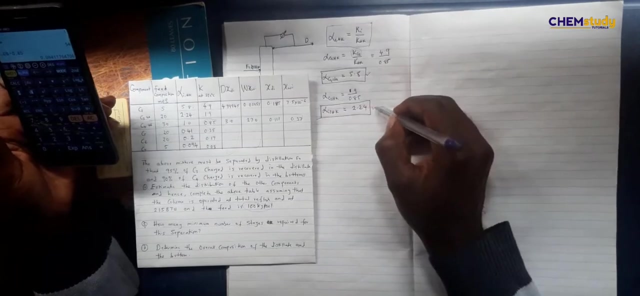 so alpha c3 hk becomes 2.24. so that's how we got the second one. so you're just writing these formats for all of them, because when the lecturer is grading your work, you would grade based on the steps and not just the table. so ensure you write out all the steps. 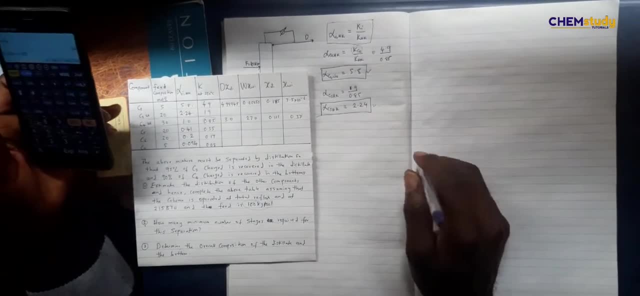 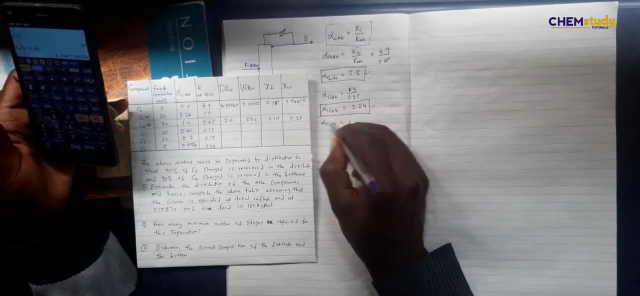 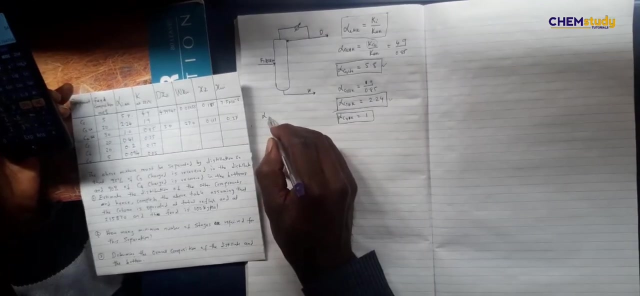 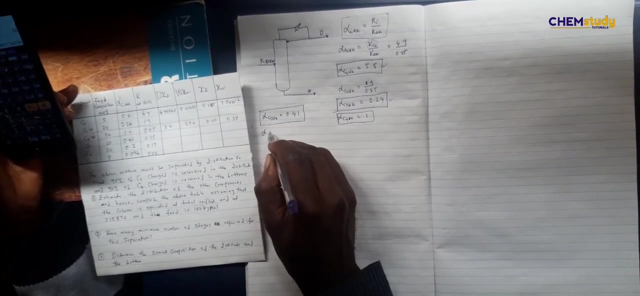 okay, so moving on. so you do that for alpha c 4 hk, which is equal to 1, then we have alpha c5 hk, which is equal to 0.41. alpha c6 hk, which is equal to 0.2. alpha c6 hk, which is equal to 0.2. 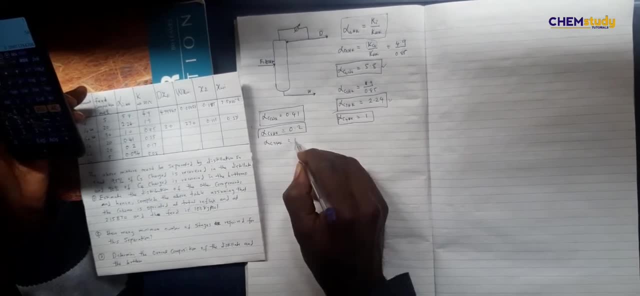 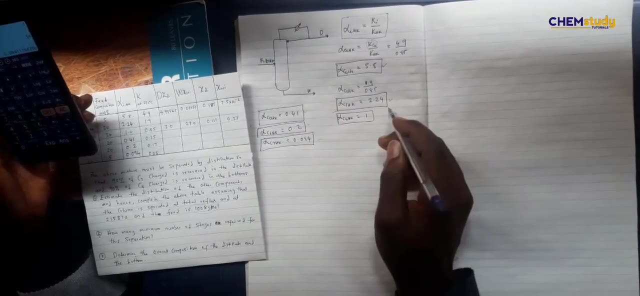 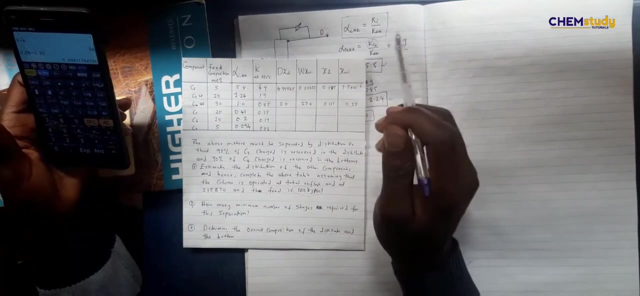 alpha c6 hk, which is equal to 0.2. alpha c7 h. then we have alpha c7 hk, which is equal to 0.094, from the cards aligned, Apple being an electronic. so you get your format and lets write it okay. so what, we are done with this first column. 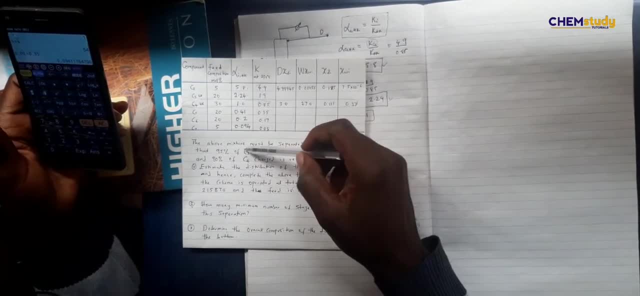 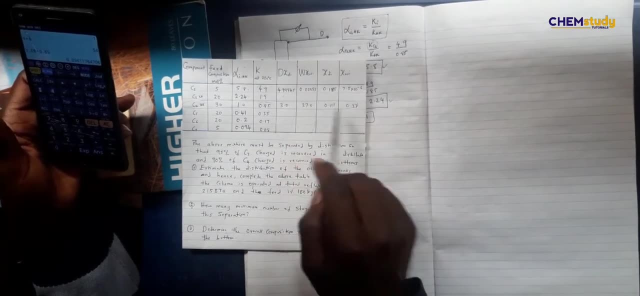 now let's look at how we can fill these. now from the question it says that ninth to five percent of see to recharge. so let's fill c3, so we will just fill them sequentially. fill them like this, like this, like this, and we vậy. 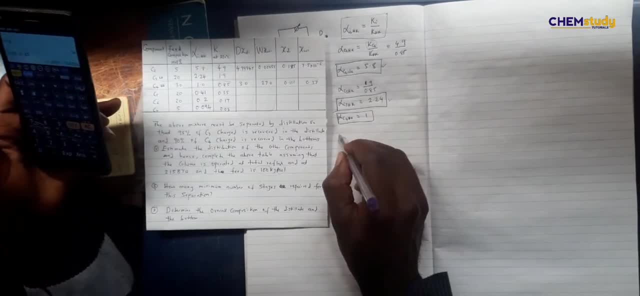 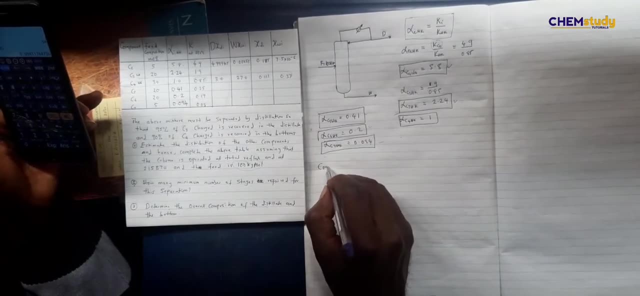 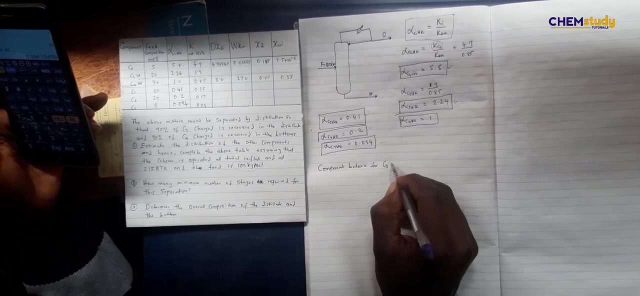 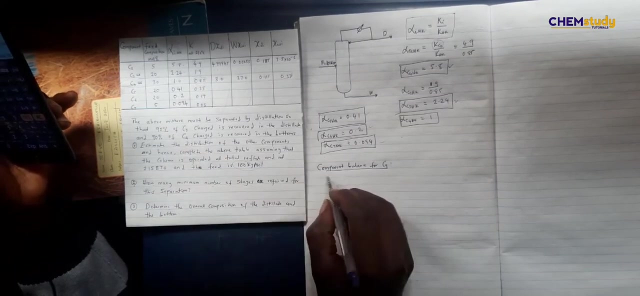 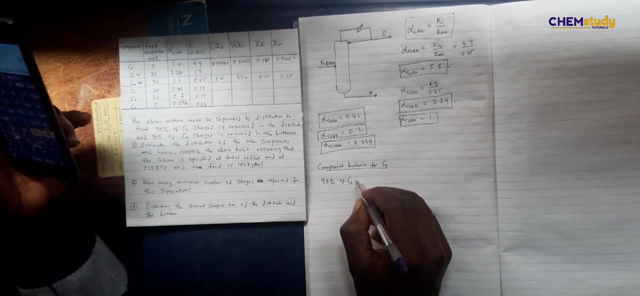 So let's find component balance for C3.. Let me shave this, Okay. So let us look at how we can do it Now. the question said that 95% of C3. Charged, meaning C3 in the feed. 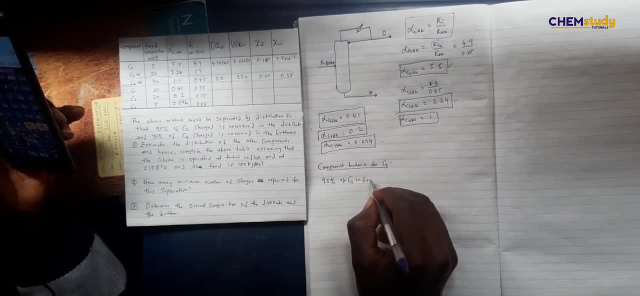 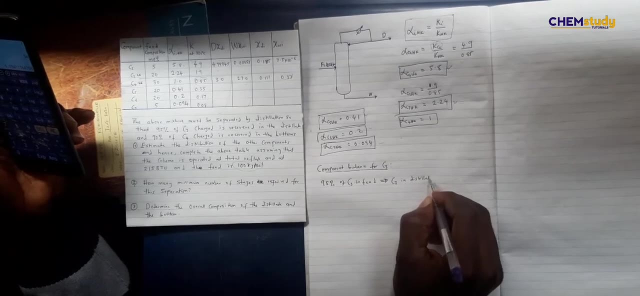 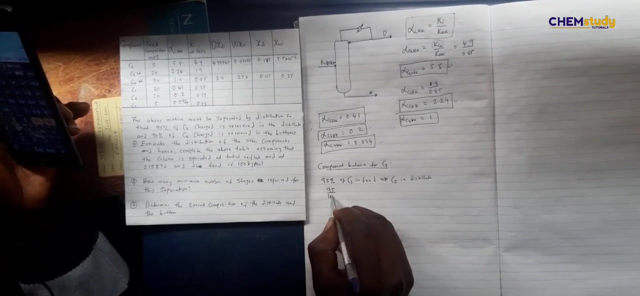 That C3 in feed is recovered in the distillate. What this means is simply: 95% is 95 over 100 of simply means times C3 in the feed. So you look at the feed. What is C3 in the feed? 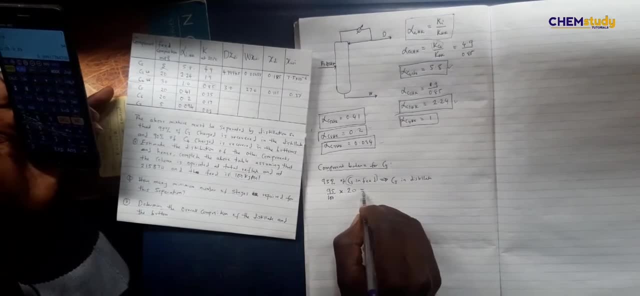 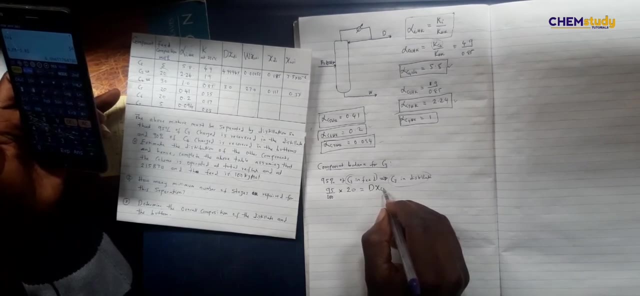 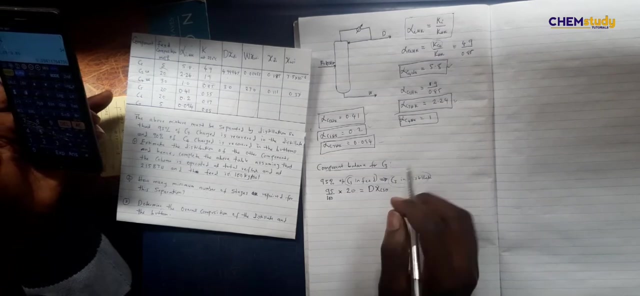 It's 20.. 20. It's equal to C3 in the distillate, That's DxC3 in the distillate. Because this is the total distillate multiplied by the fraction, You get the total value of C3 in the distillate. 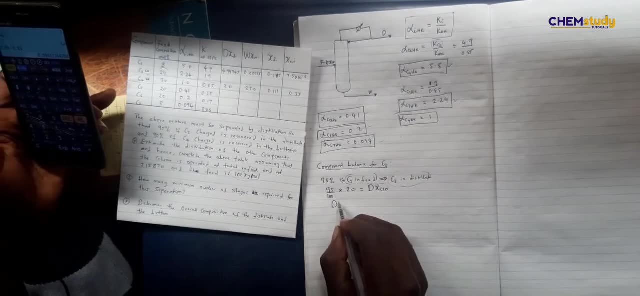 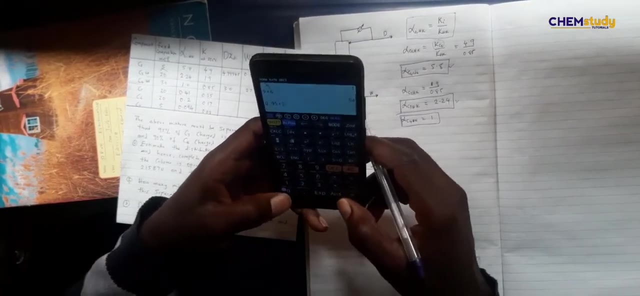 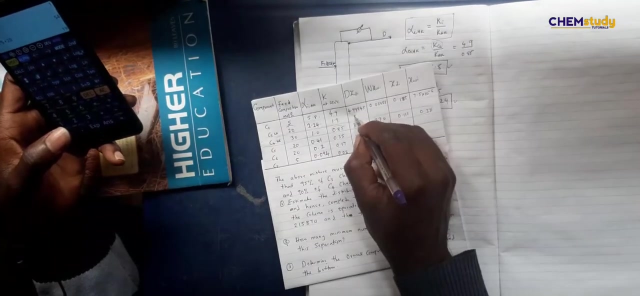 So this becomes. So. if we make this subject of the formula, DxC3D, becomes 0.95 times C3. It becomes 95. So this becomes 19.. So this becomes 19.. So you see how we are filling our table, one after the other. 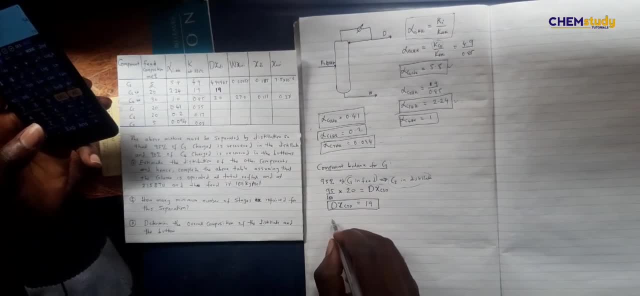 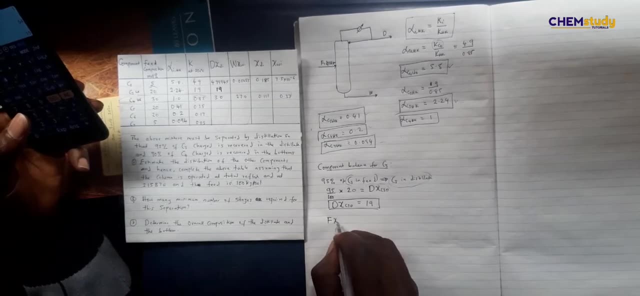 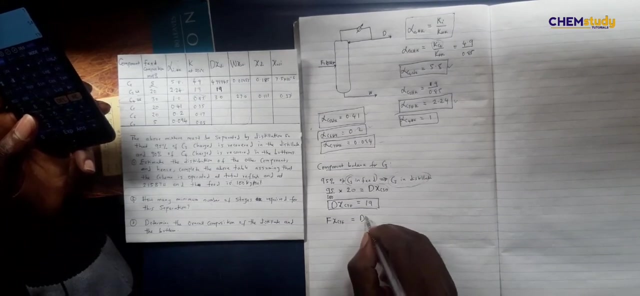 Now also component balance for C3.. We know that C3 in the feed, Which is C3 in the feed, Which is FxC3 in the feed, Is equal to C3 in the distillate Which we just found. 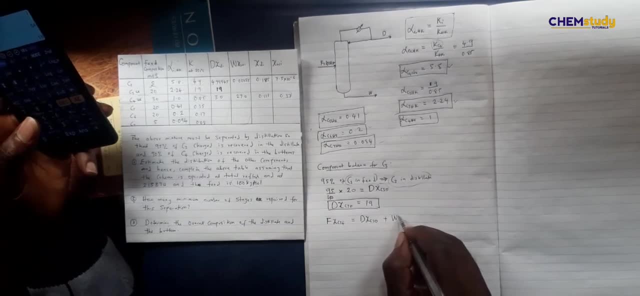 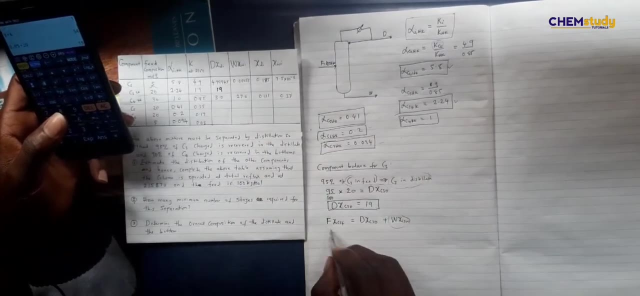 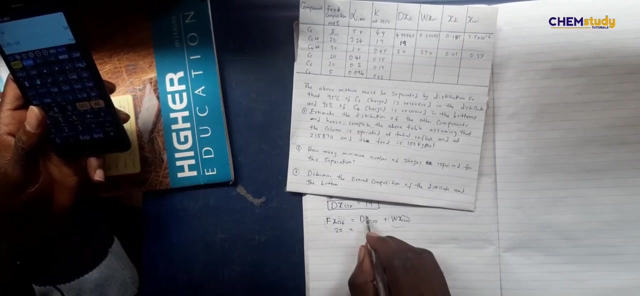 XC3 in the distillate, Plus C3 in the waste. Now we are looking for C3 in the waste, Which is this one. So this one is FxC3 in the feed Is 20.. So we have 20 is equal to. 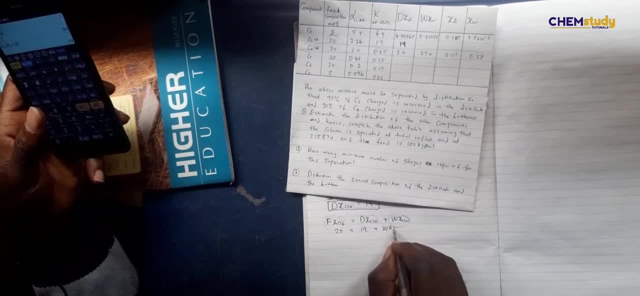 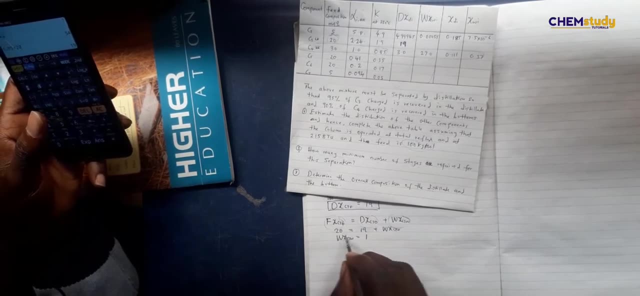 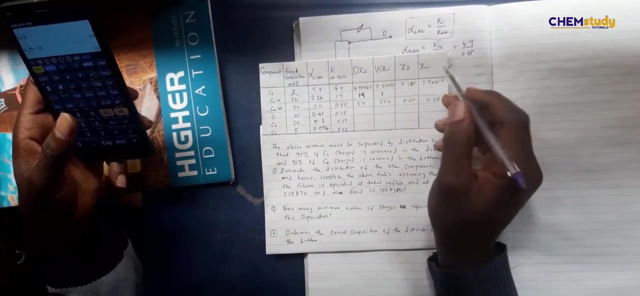 We just found this one to be 19.. Plus So C3 in the waste becomes 20, minus 19 is 1.. So we found this, Which is 1.. Now to find XDI. If D, XDI is 19.. 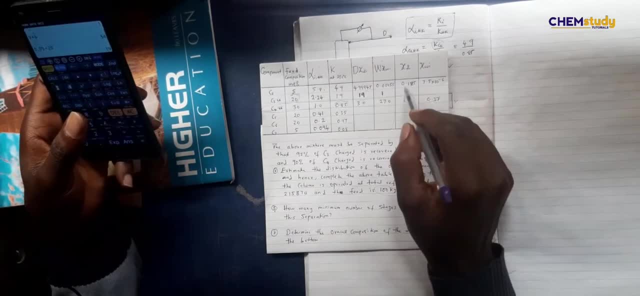 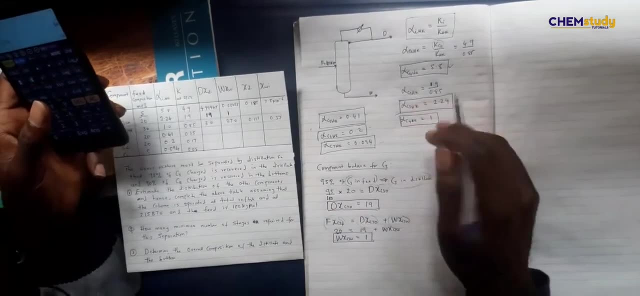 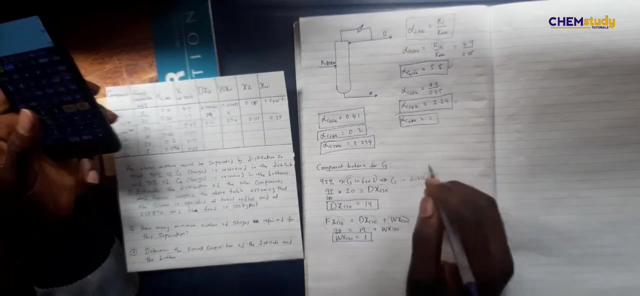 Okay, If we can find the value of D, They would be able to find XDI. So how can we find the value of D? We would have established this initially. So let us establish a value for D. Okay, Okay. 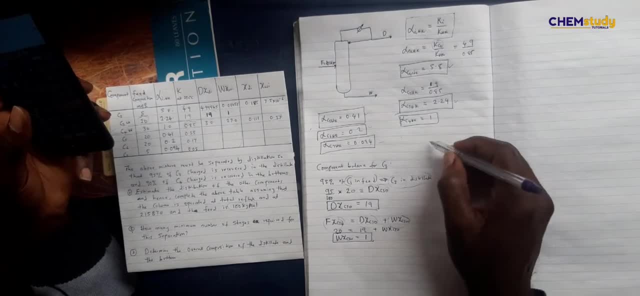 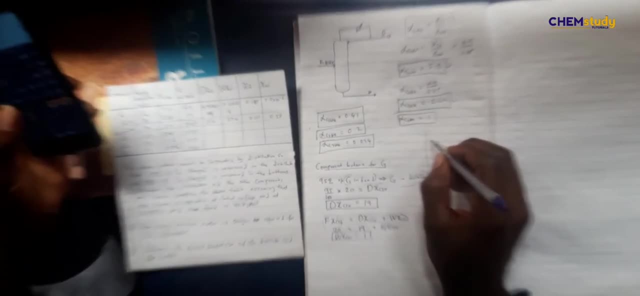 So how do we do this now? Let me just draw a separate column. So this should be one of the first things you would establish. Let me draw a separate column Now, if you look at C2. C2. Okay, 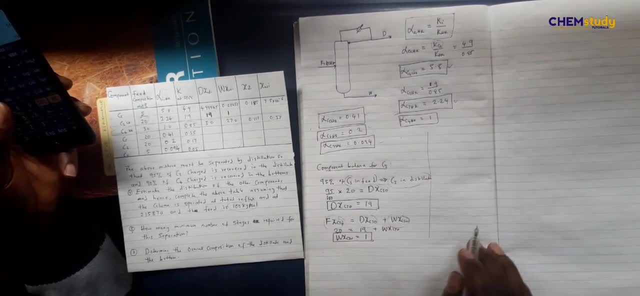 Let me just continue from here. Let me just Let me continue from here. Okay, Since this is a different component, Let me just do it from here Now. if you look at C2.. Let me bring the question closer. You would see that. 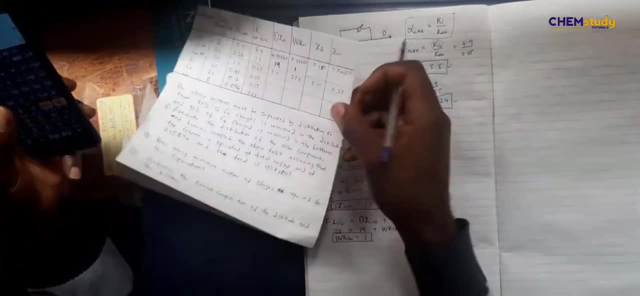 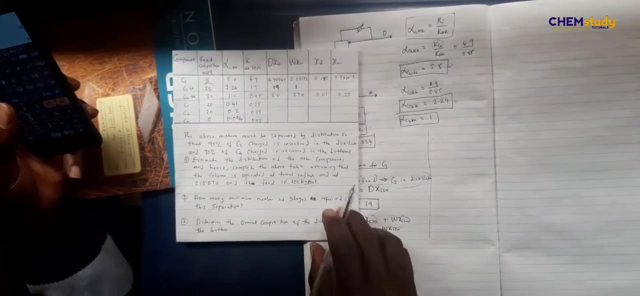 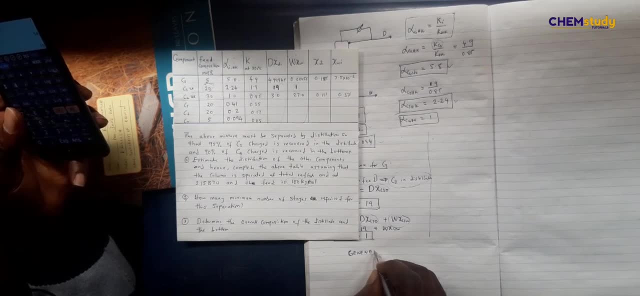 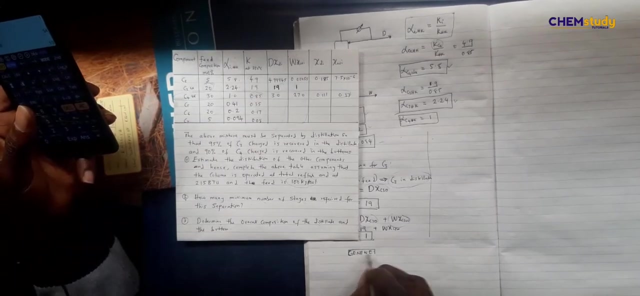 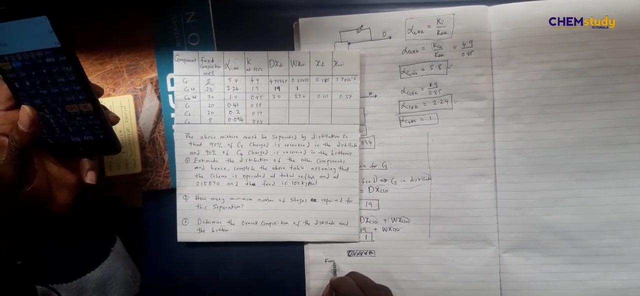 Okay, We could still get it from C3.. I am trying to look for the easiest way we could do this. I am trying to look for the easiest way we could do this. Okay, Okay, there is no need to even have a general mass balance now from from c2, from c2. 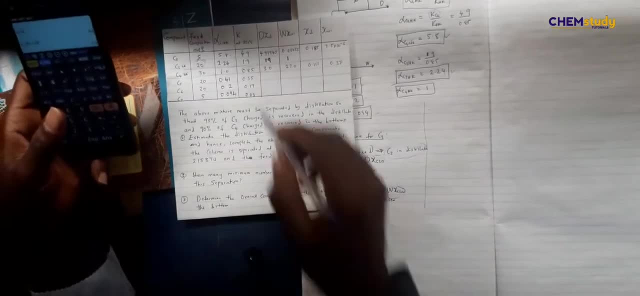 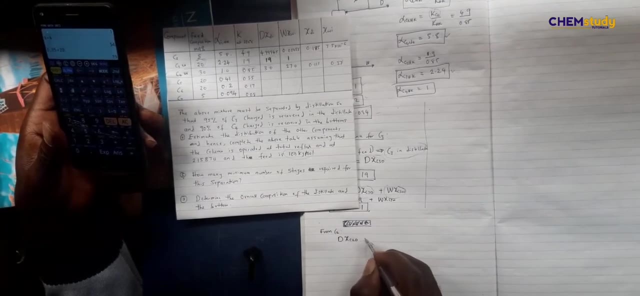 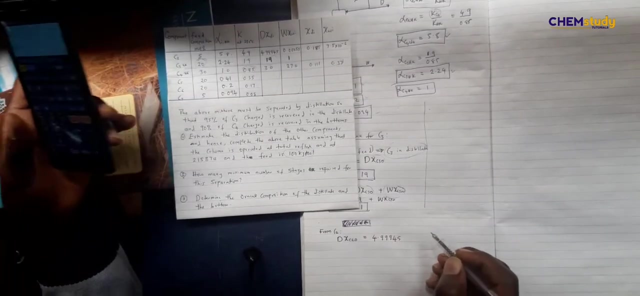 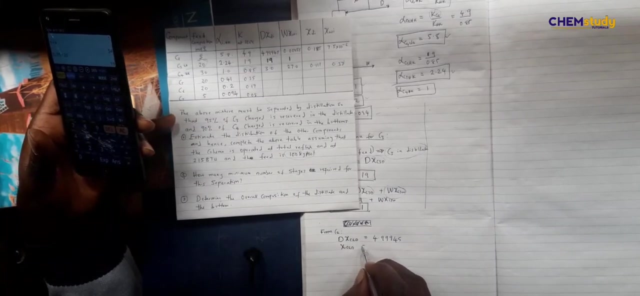 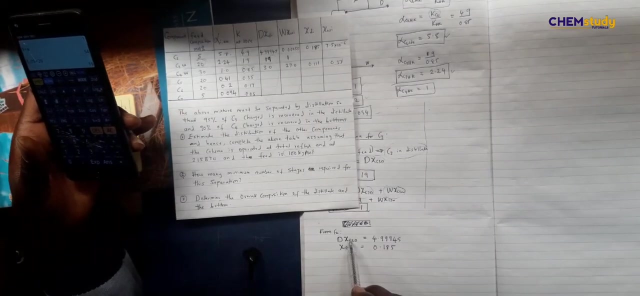 see, this is capture okay from c2, dx. so dx c2 in distillate is equal to what? four points, four, point nine, nine, nine, four, five, okay, now x of c2 in the distillate is equal to what? from this column we have 0.185. so if d times this gives this and only x, c2. is this so to find d? 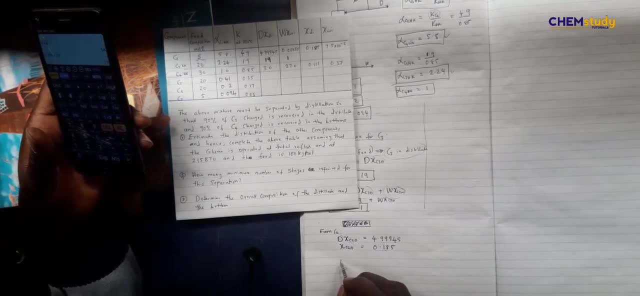 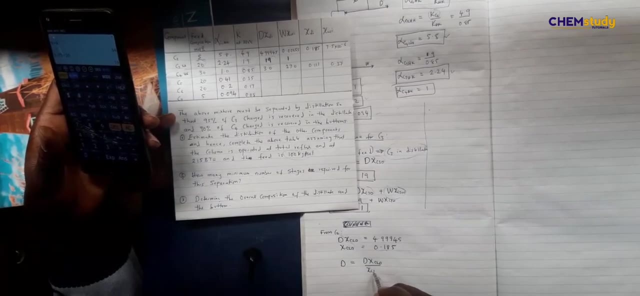 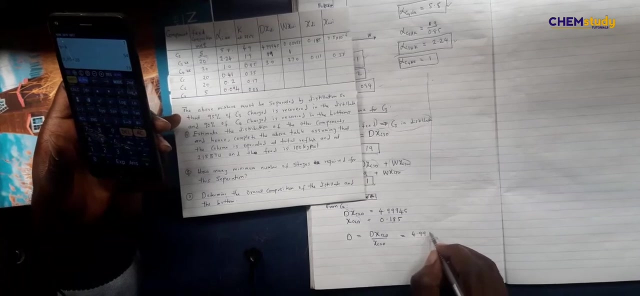 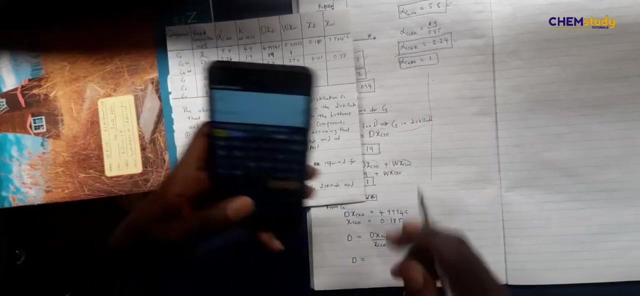 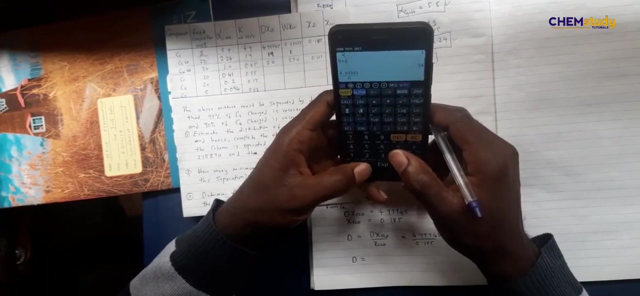 you simply divide this by this, so it means that d becomes d x c2 in the distillate divided by x c2 in distillate. okay, so which would be 4.99945 divide by 0.185. so d becomes- we use our calculator- 4.99945 divide by 0.185. 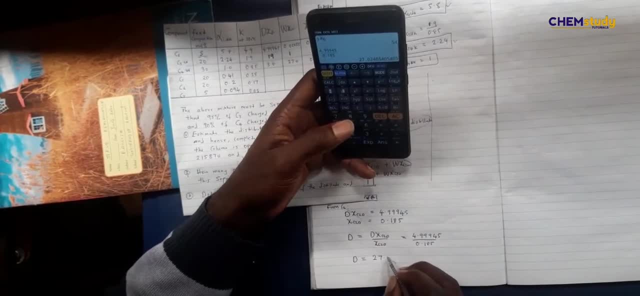 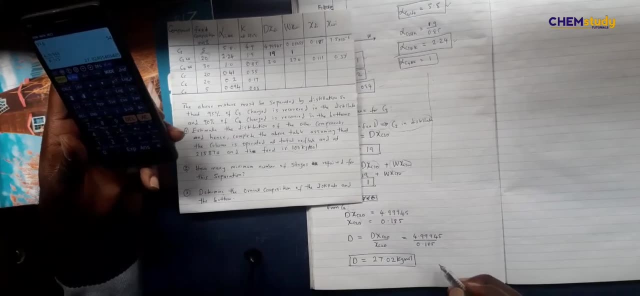 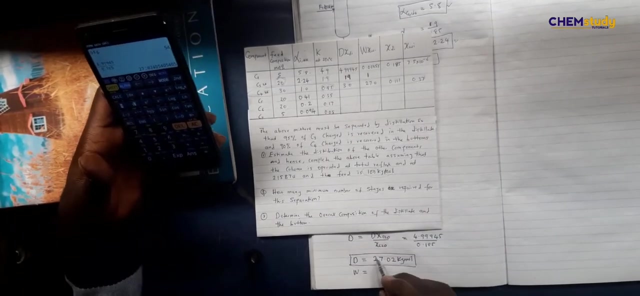 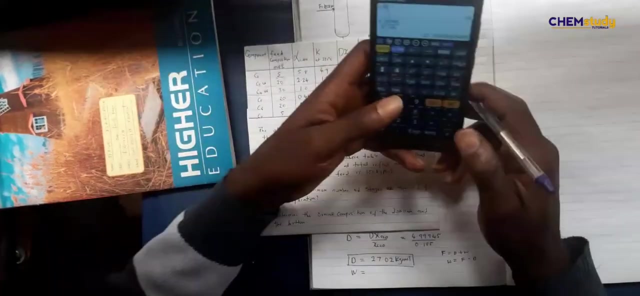 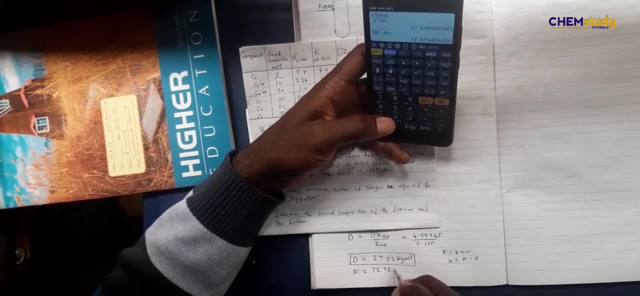 so half 27, half 27.02 kilogram more. okay, now, if your feed is 100 more, this means that w becomes 100 minus this, because p is equal to d plus w. so w becomes feed minus distillate. so that is 100 minus this later 72.98. 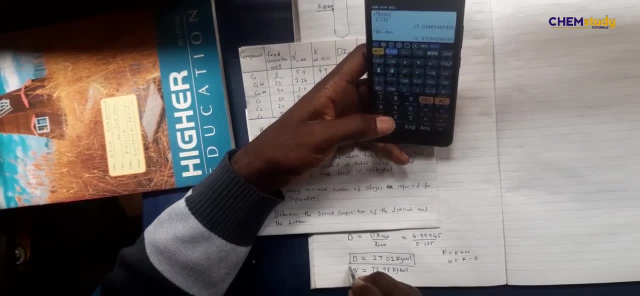 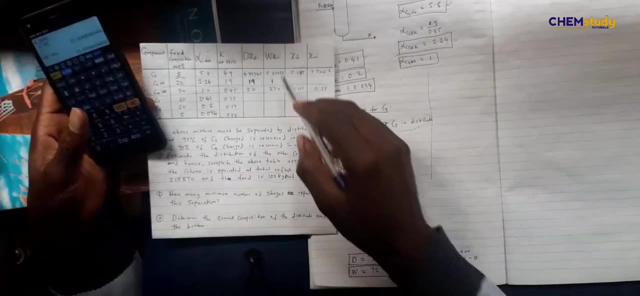 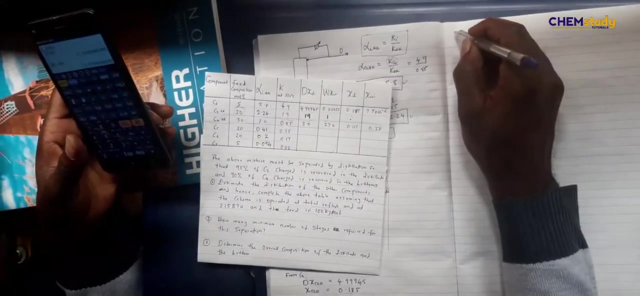 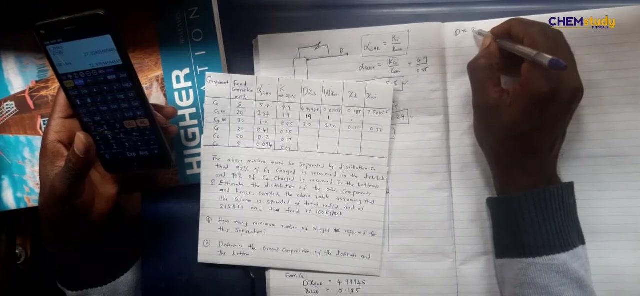 programs. so that is the bottom struggling. so we would need this noun to calculate x, d, i. so, um, if d is equal to 27.02 and d is equal to 21.6, and this one because if d times a is equal to 22.、. 0.2 and d is equal to 67.02 and you can come back. so if red means d, então buçuk, Maria for蒲, and blue means stay away, final result. so if we see here we have b, the river, this volume, so this contents we want to know here, so that therefore, 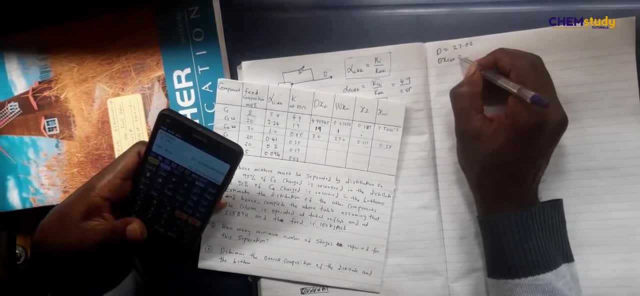 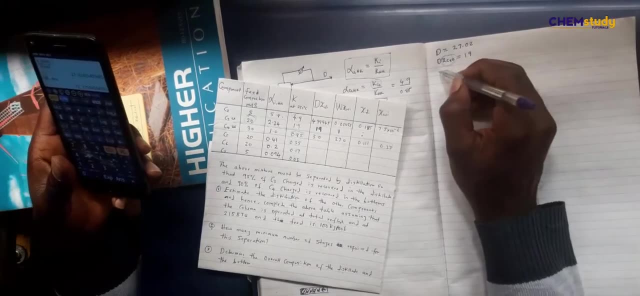 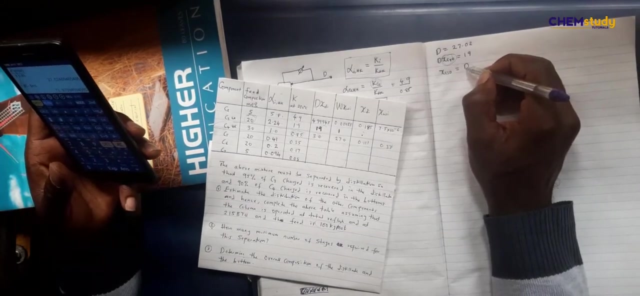 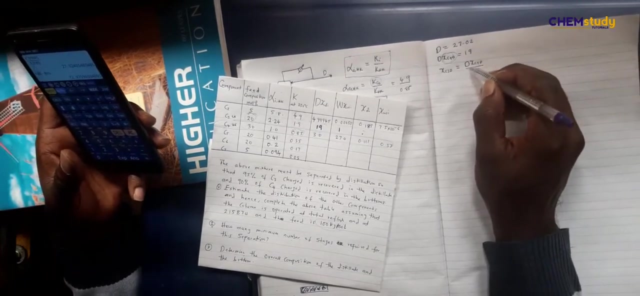 xc3 in the distillate is 19, so we can find xc3, the fraction of xc3 in the distillate, the fraction xc3 in the distillate becomes. it simply becomes d xc3 in the distillate divided by you. divide by d, so that when d 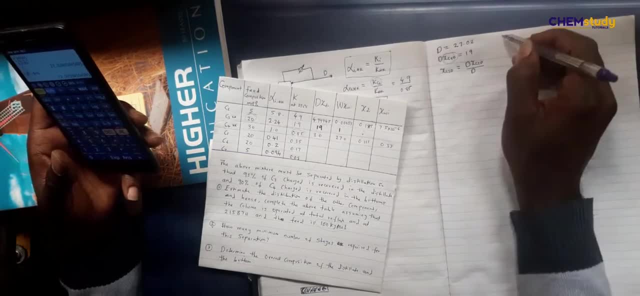 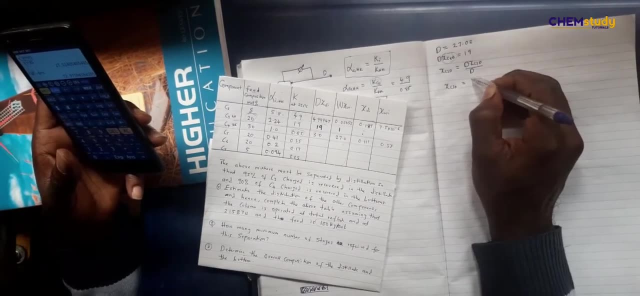 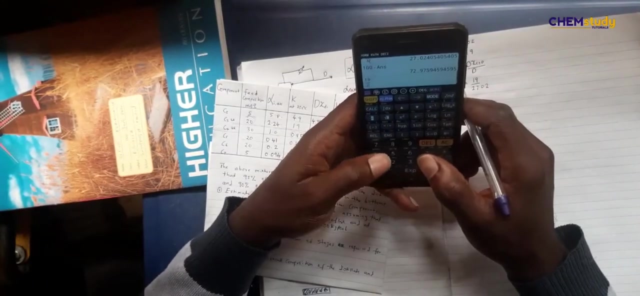 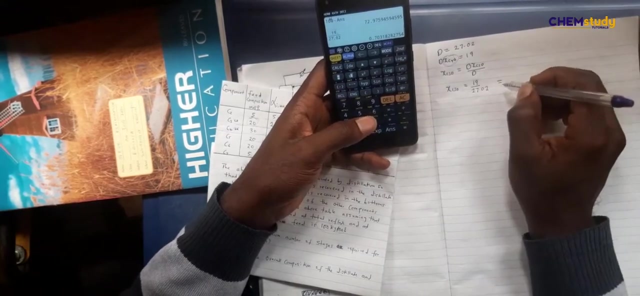 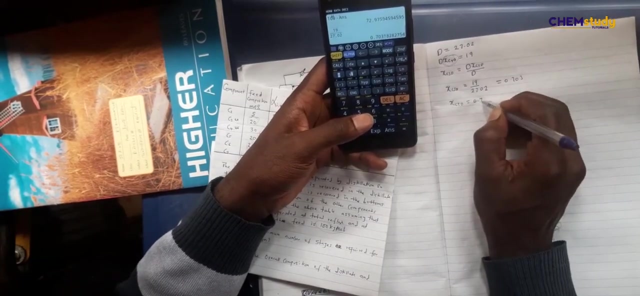 cancels the. you've left with just the fraction. okay, so xc3 in this list becomes 19 over 27.02. 19 divided by 27.02, that's 0.703, so 0.703. so xc3 in the distillate is 0.703. 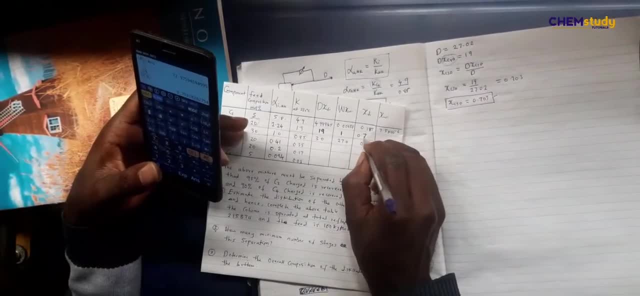 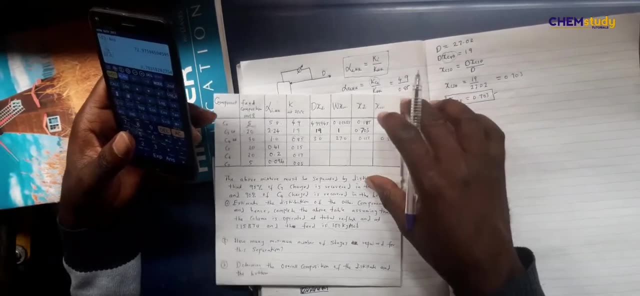 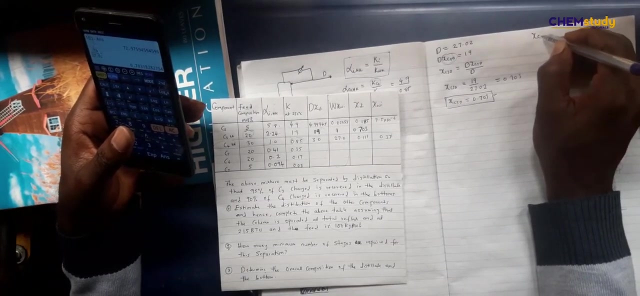 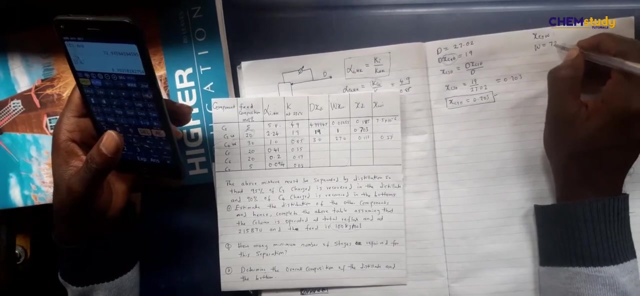 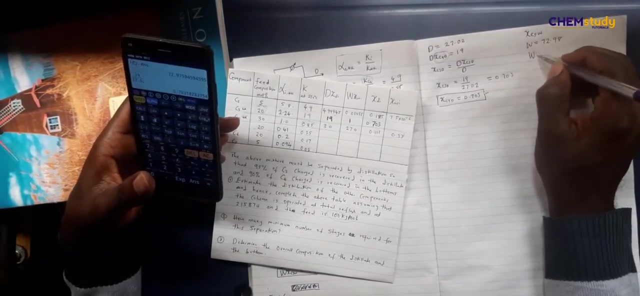 so we found another, so this is 0.703. okay, so now to find xwi is the same thing, that's xc3w. so to find this, you know that the w is 72.9, it's calculated, that's already here and w xc3w from our table is 1. 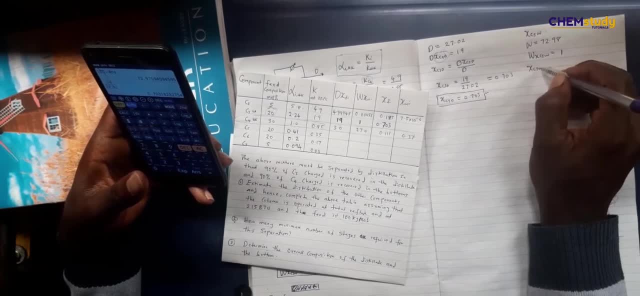 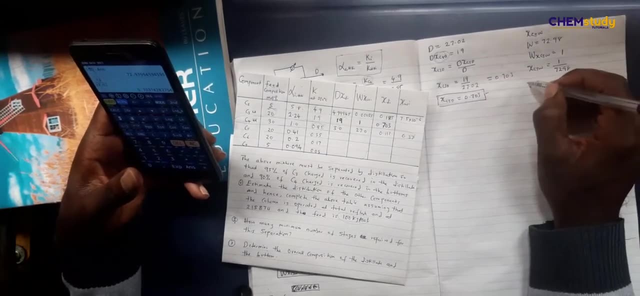 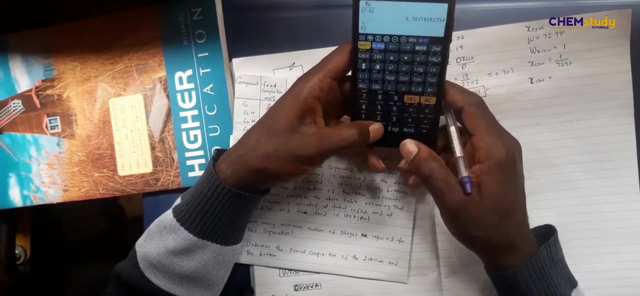 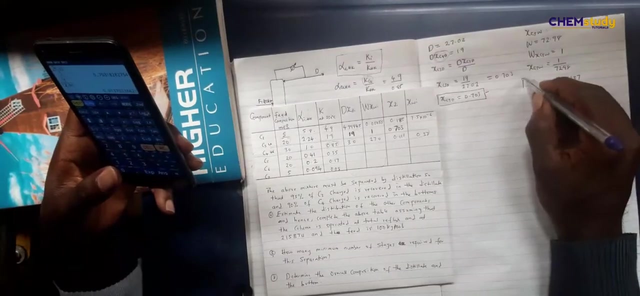 that means that the fraction xc3w becomes 1 over 72.98. it's just the same way we solve this so that xc3w becomes 1 over 72.98. that's 0.0137. so we found another 0.0137. 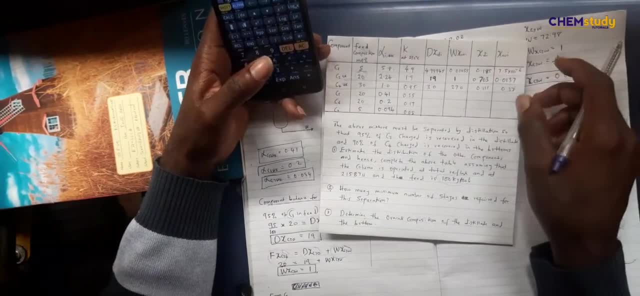 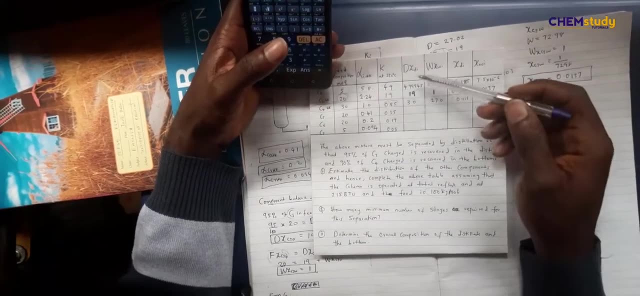 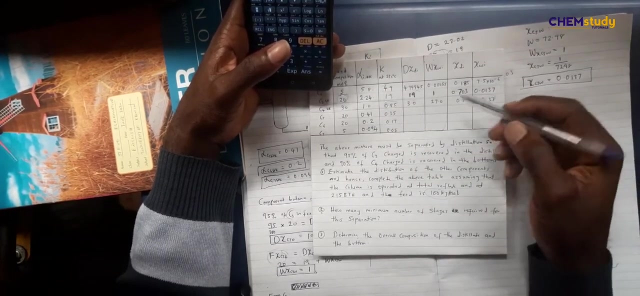 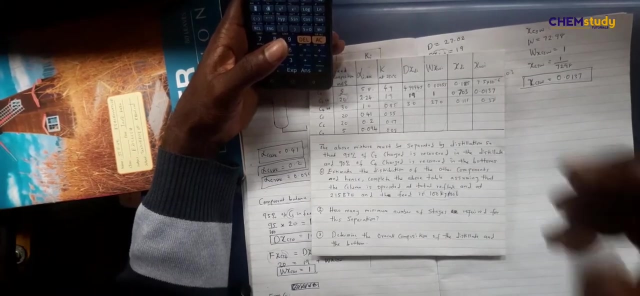 so you see how we filled this row very easily. now the next thing we want to do is to fill these orders. we do not have any detail. we do not know the distribution in the distillate for c5, c6 and c7. neither do we know the distribution at the bottoms. so we need two equations. but let's just. 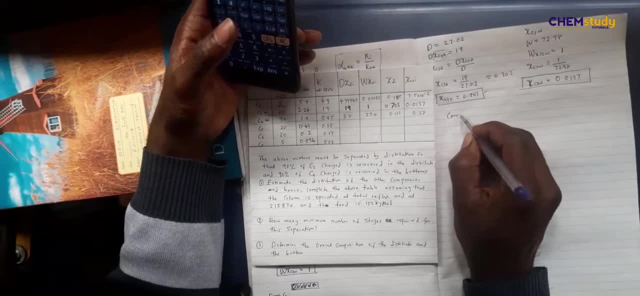 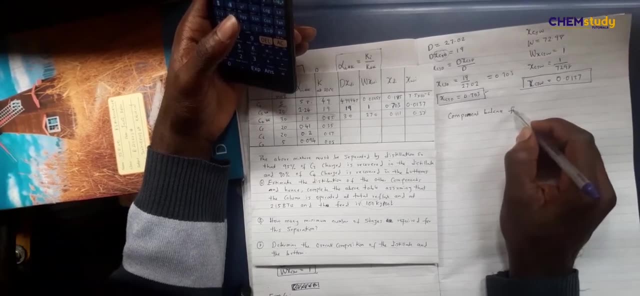 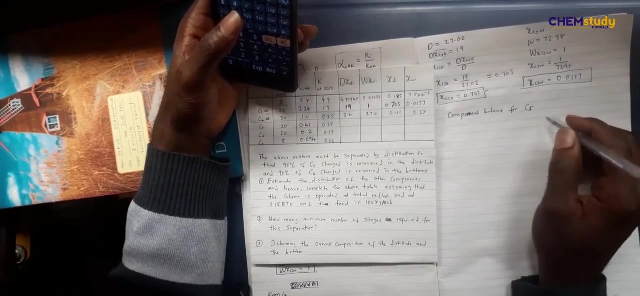 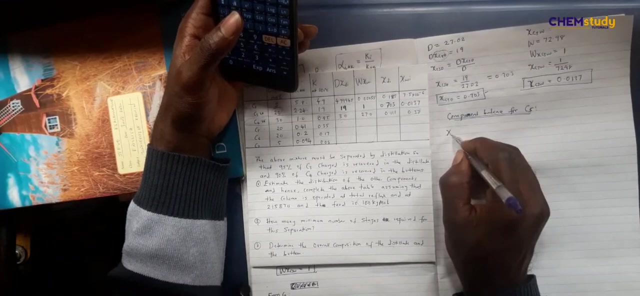 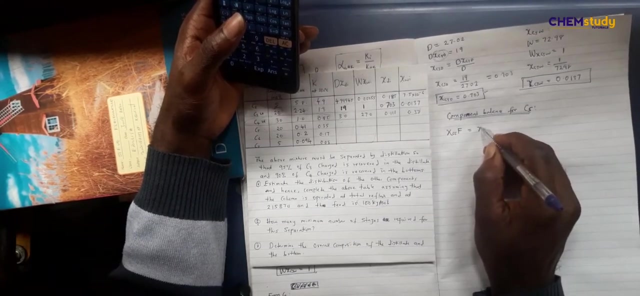 proceed now components. so we are done with c3. now component balance for c5. so one of you: c5, c6 and c7 for c5. now now you know from component balance, x of c5 times the feed is equal to x or c5 in the feed times the feed. so what's the x of c5 when? 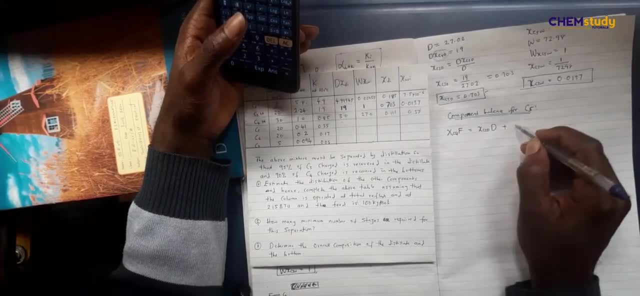 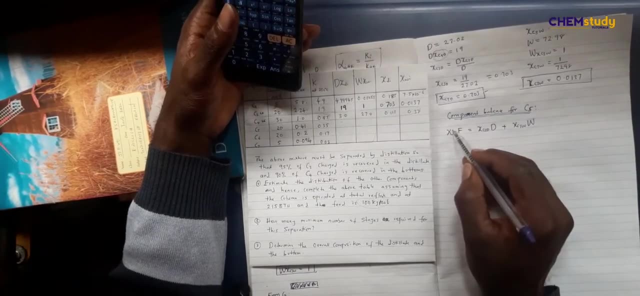 it distillate, the fraction of c5 in this times the distillate, plus the fraction of c5 at the bottoms times the bottoms. okay, now, what is everything here? the total amount of c5 in the distillate data, every thing here, the total amount of c5 we use here, So that change on the身 jumple sin igual plus. 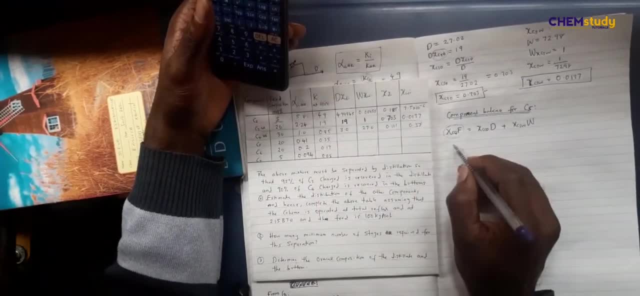 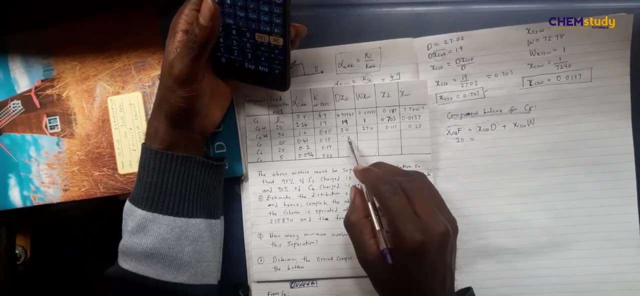 in the feed is 20, so we have it as 20, equal to total amount of c5 in the distillate. okay, we do not know it, but we know the value of the distillate, so let's write this so: x c5 in the distillate. 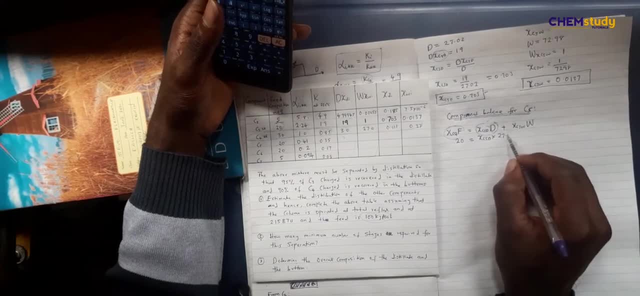 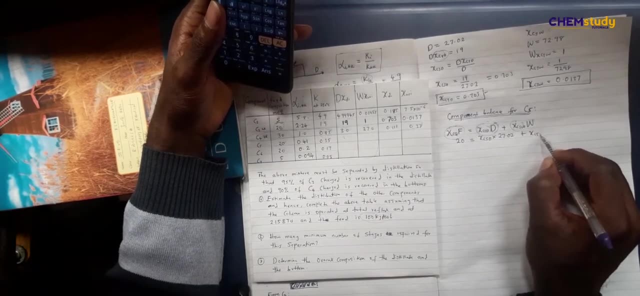 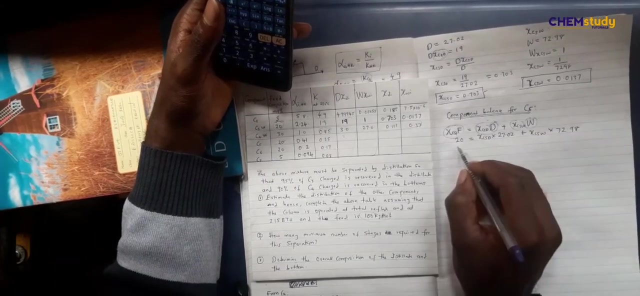 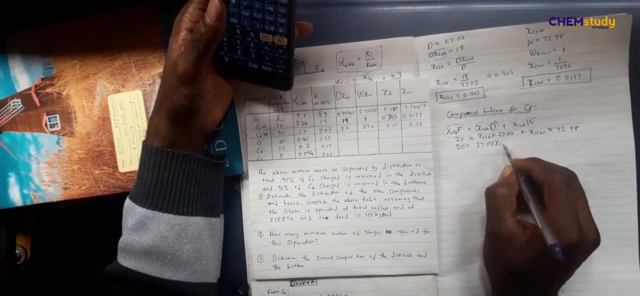 times what is distillate 27.02 plus x c5 w? we do not know it, but we know the waste as 72.98. so we have an equation: 20 is equal to 27.02 x c5 in the distillate plus 72.98 x c5. 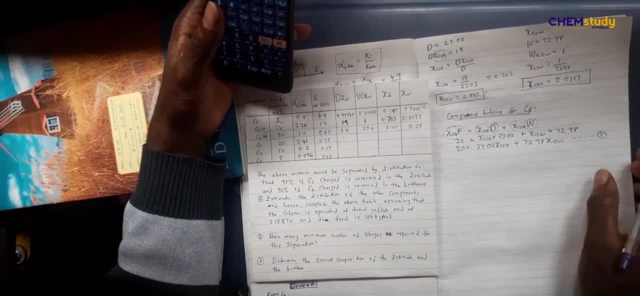 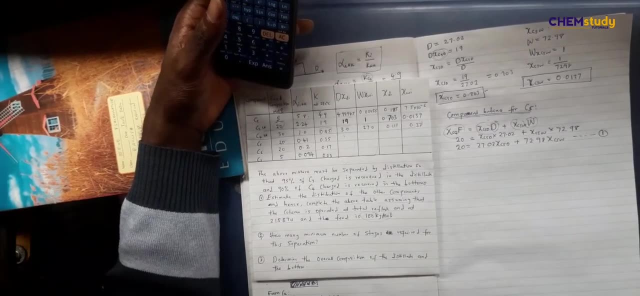 so this is equation one, so we need a second equation. we need a second equation to be able to solve it, because we have two unknowns. so we need a second equation. we need a second equation to be able to solve it, because we have two unknowns. 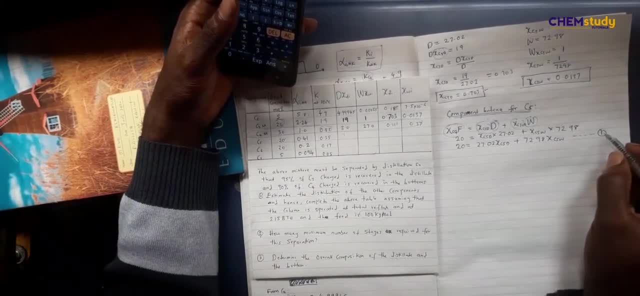 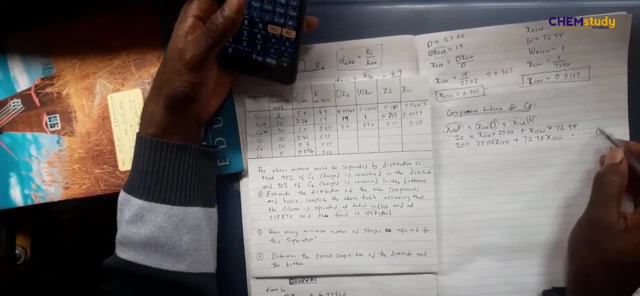 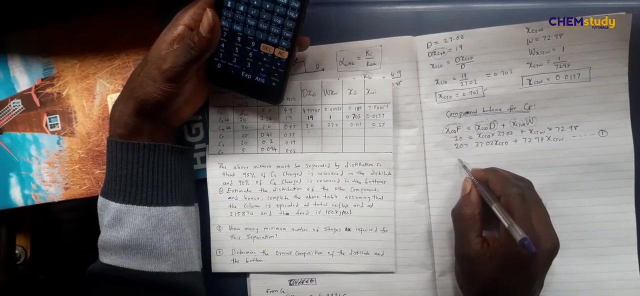 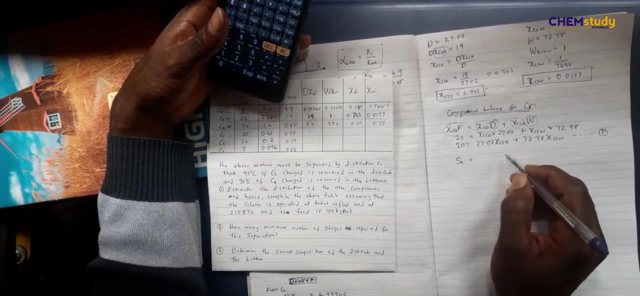 one equation, so we have to come up with a second equation. so how do we do this? there's an equation called fenske equation which goes like this: s of a component, let's say e, is equal to relative volatility of e with respect to a heavier component. 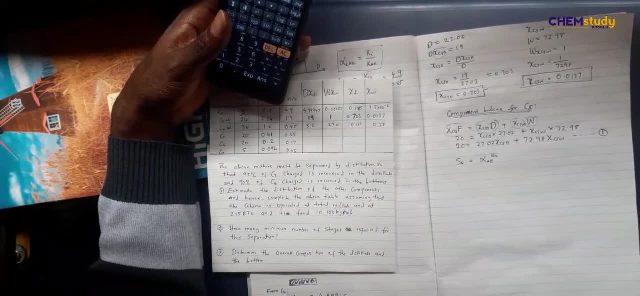 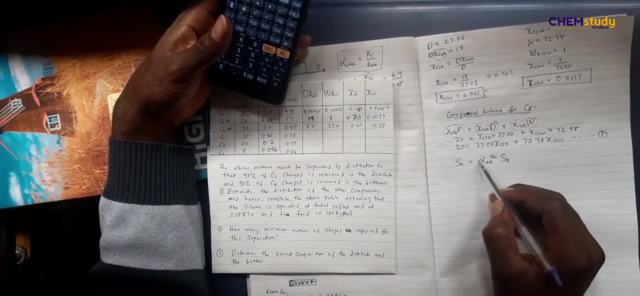 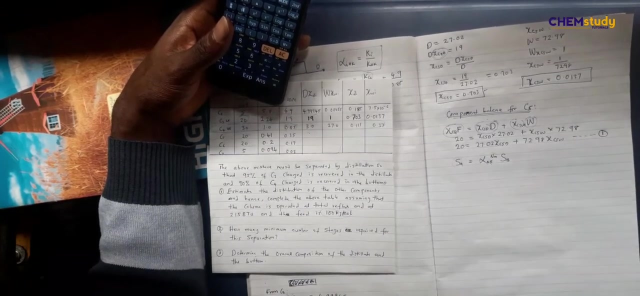 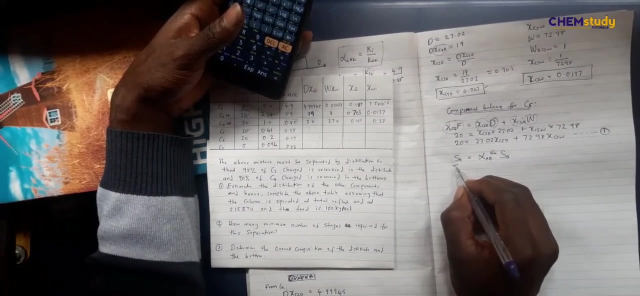 times the minimum number of stages s of the heavier component, so s of a lighter component is equal to the relative volatility of the lighter component to the to a heavy component, which is the power of the minimum number of stages times s of sb. now let me define these terms: s e. 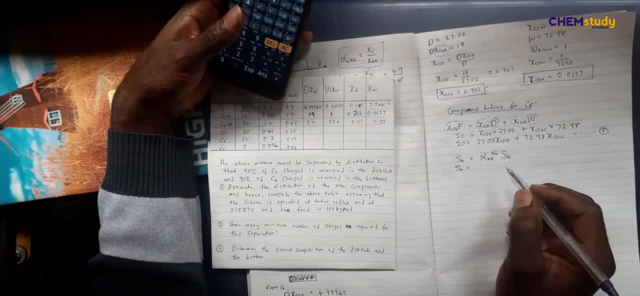 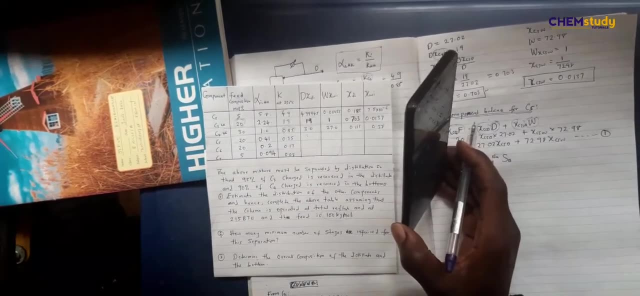 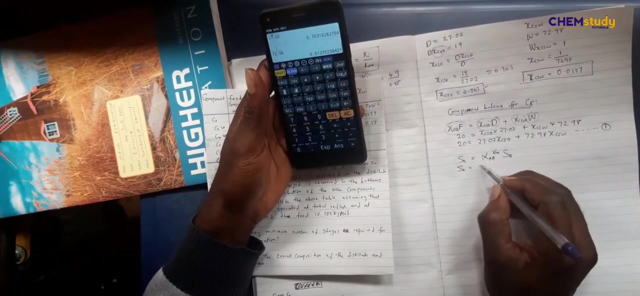 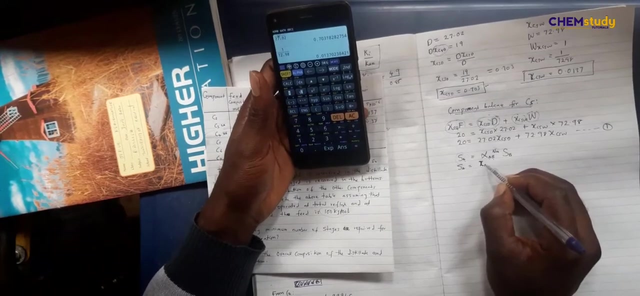 er, s e okay. x is simply it's. it's a term which um simply means right the okay, because s s x of e in the distillate. so it's called it's only split. so it's called it's just it's split. s p's no school, it doesn't start after adventure. but we know it. it that's what we do. one little频c 나는. 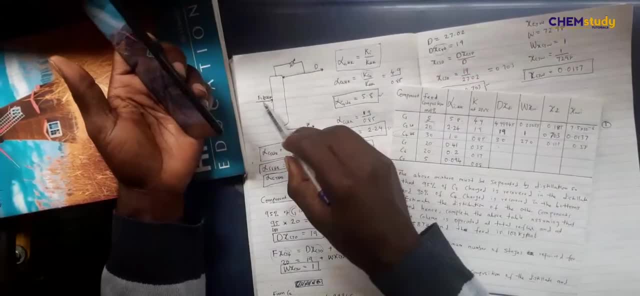 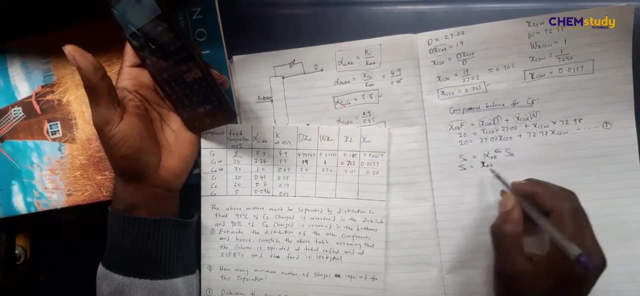 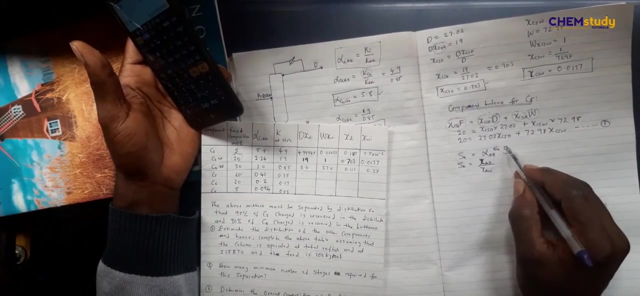 version shows the split, how it splits, how the component splits, from the feed to the distillate and the waste. okay, so it's the ratio of the distillate fraction distillate to the fraction at the bottoms, x a d over x a w. so that gives the split. y s of b is equal to x. 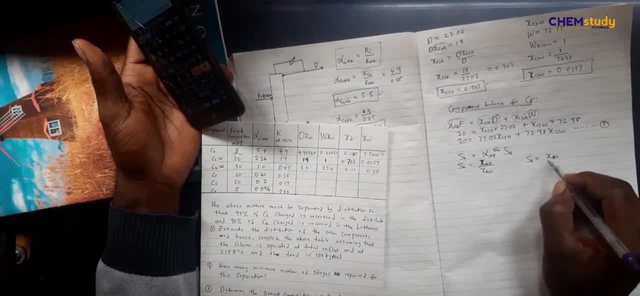 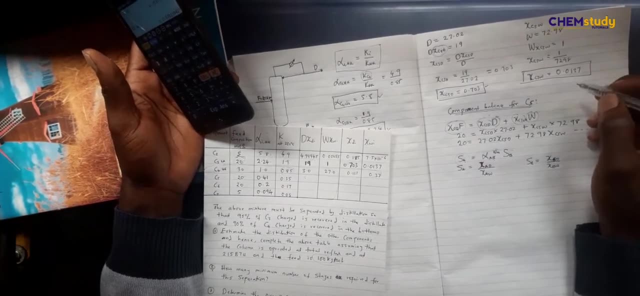 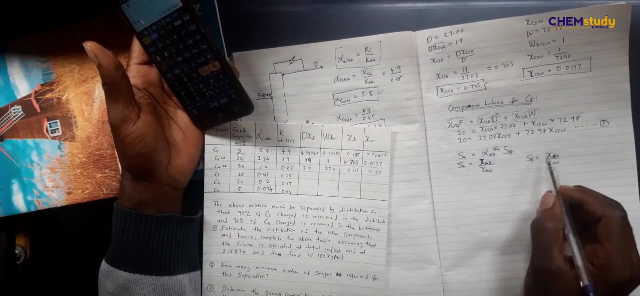 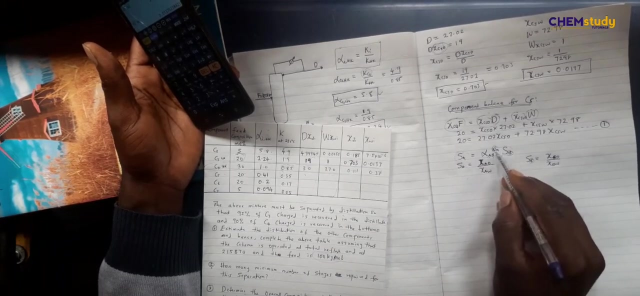 b d over x b w. okay, that's how you get this place. remember, like i said, this time around our heavy key, our heavy key will take the place of sb. so whenever we see b, we put a heavy key. okay, so take note of that. so this becomes um, so let's make n in the subject of the formula. like i said, this is fenske equation. 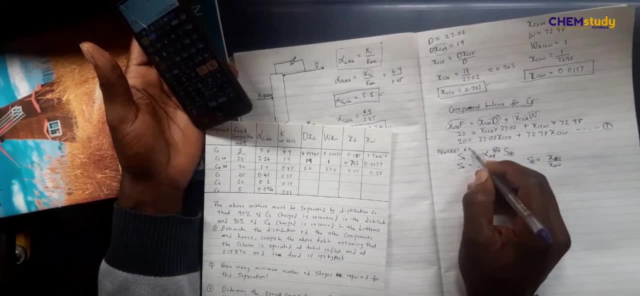 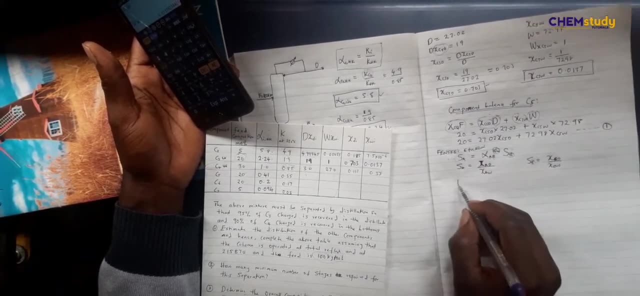 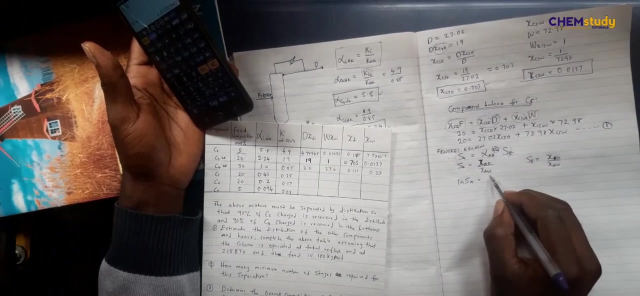 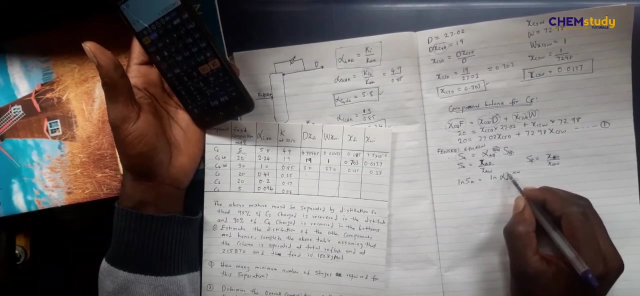 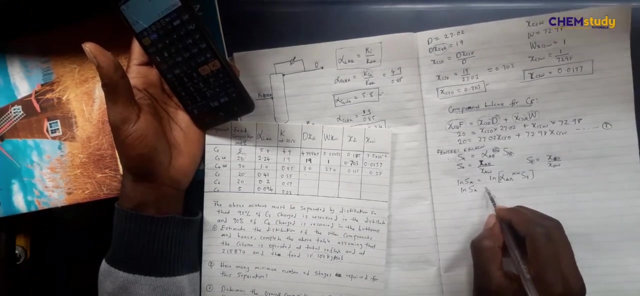 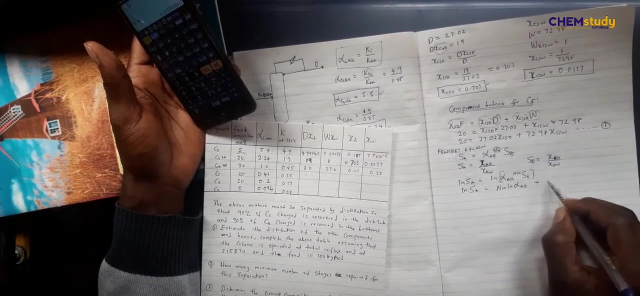 fenske's equation. now, if we are to make nm the subject, if we take lean of both sides, so lean s a would now would be nm could come down. okay, let me just write it fully for those who may not understand. so you for to open the lane. this becomes nn, lane a b plus lean s b. okay, if we 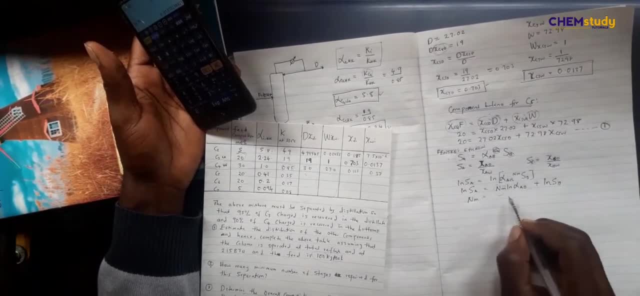 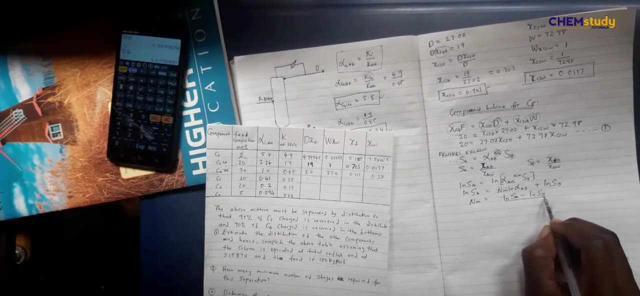 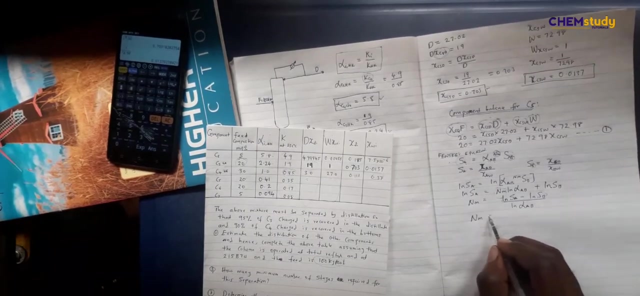 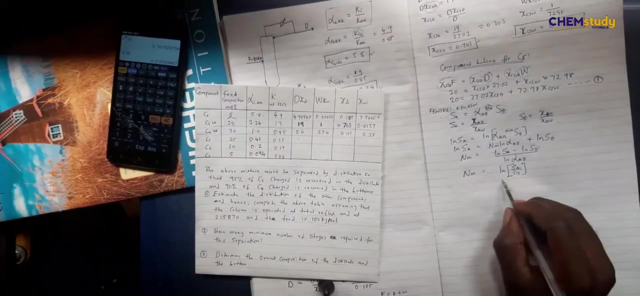 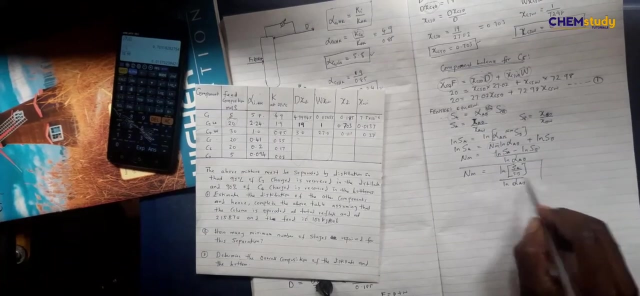 make nn the subject of the formula, nn becomes lean s a minus lean s b over lean a b. if we are to further simplify this, this becomes lean s a over s b over the relative volatility of a with respect to b. so this is the formula we'll be working with. 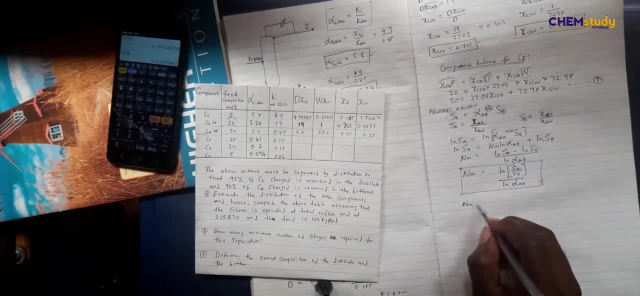 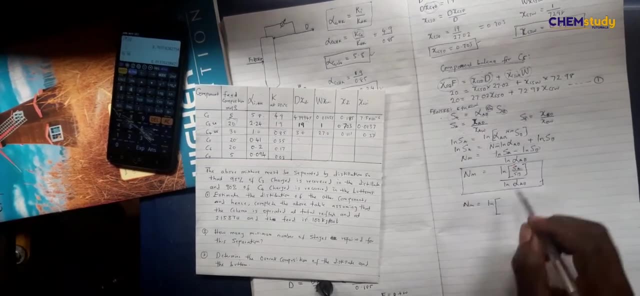 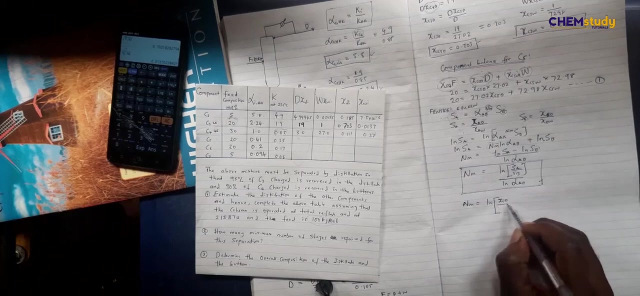 let me put the values of s a, so n m becomes lean. what's s e? we defined it. let me just use i. so this is x of i in the distillate over x of i at the bottoms. now divide by. so let me divide by sb. remember that sb, like i said, is the heavy key. 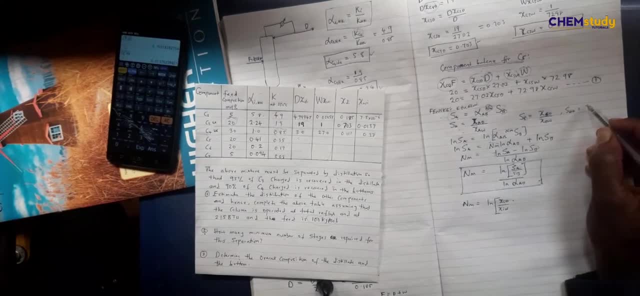 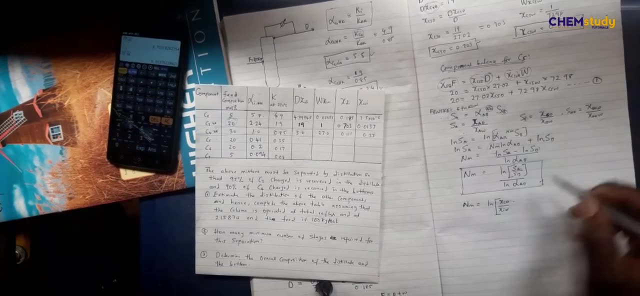 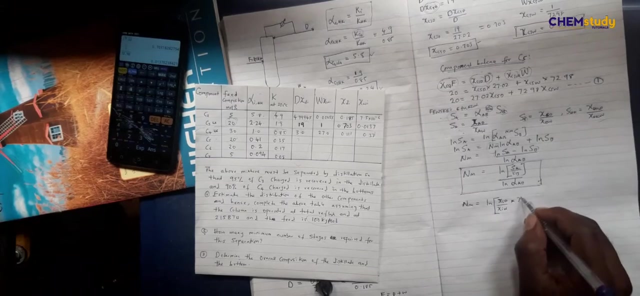 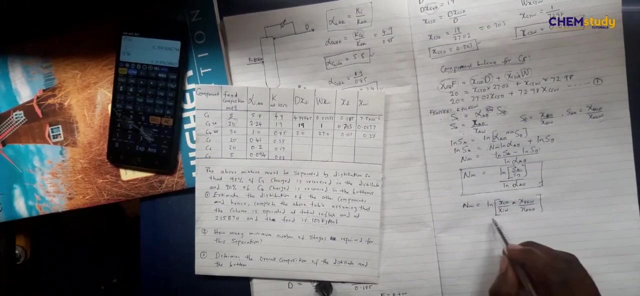 so that is s heavy key becomes x of heavy key distillate over x of heavy key and the way that is split. so if we are dividing this, if we're dividing this, i want to use product here as time. so x of heavy key w over x of heavy key in this leaf. this is what we have over relative volatility of. 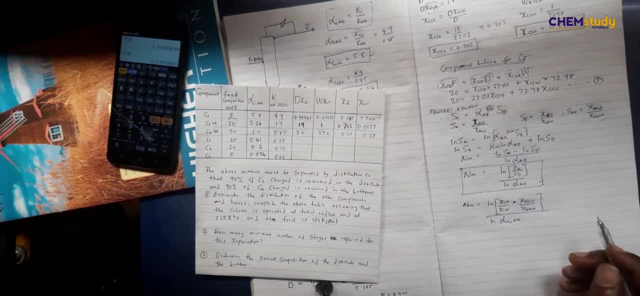 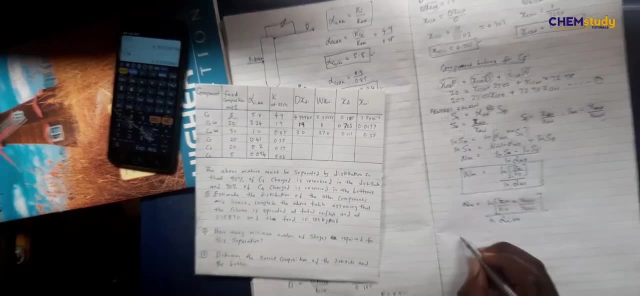 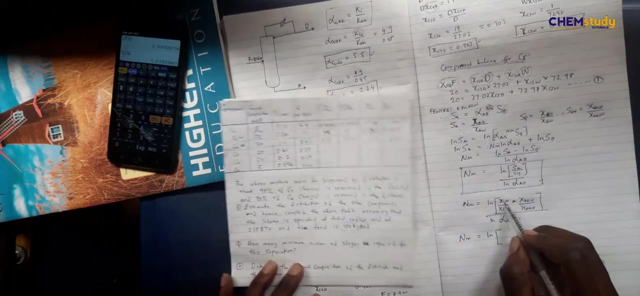 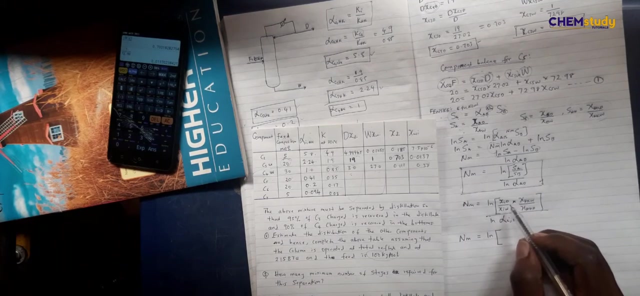 lean i heavy key. okay, so we just replace b with heavy key. so we just replace b with heavy key. so we just replace b with heavy key. so n m becomes lean. what is x of um the i we are working with now? okay, we could in fact, as a matter of fact, at this point, since we're looking for the minimum, 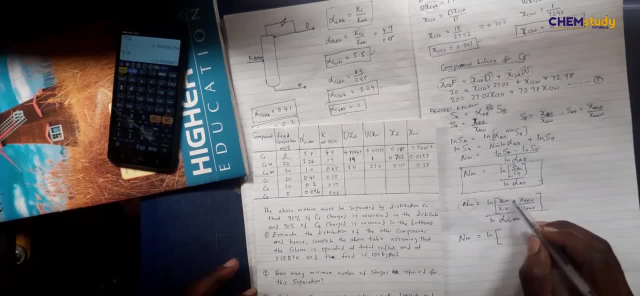 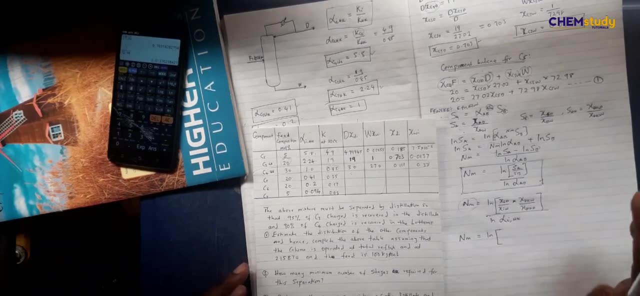 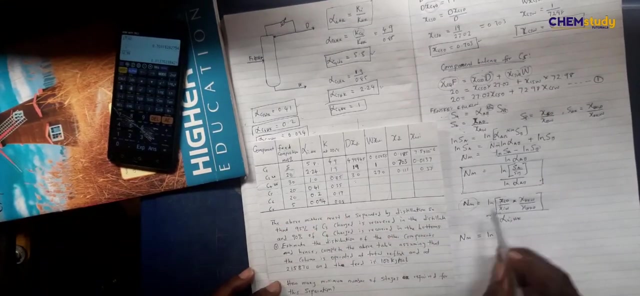 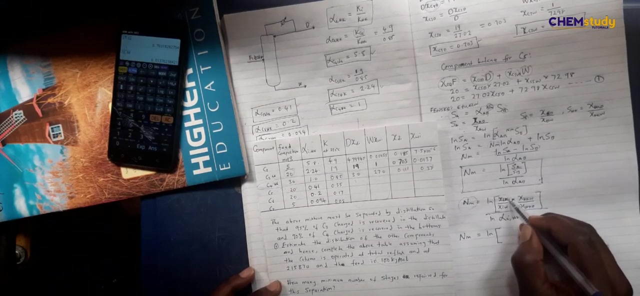 reflux. we should. we're working with light key. yes, light key and heavy key. please take note of that: light key and heavy key. so this our i should be our light key in. yes, exactly so, um x id, because it was a light key, light key distillate, so you could change this to lkd l k, d, l k w. so what's? 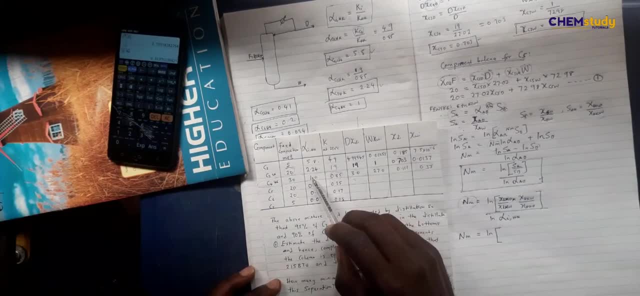 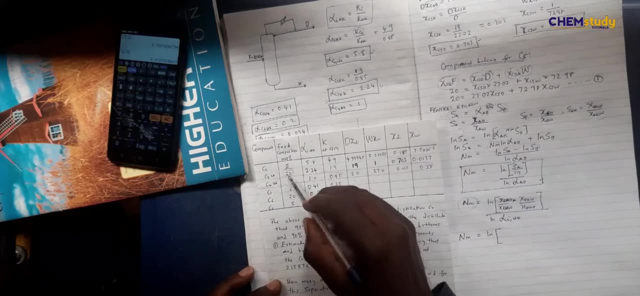 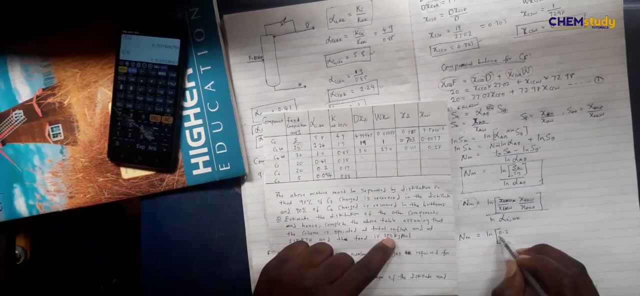 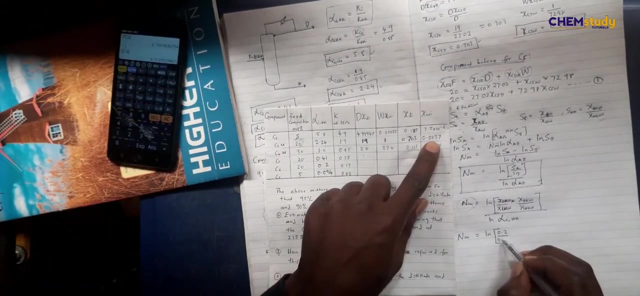 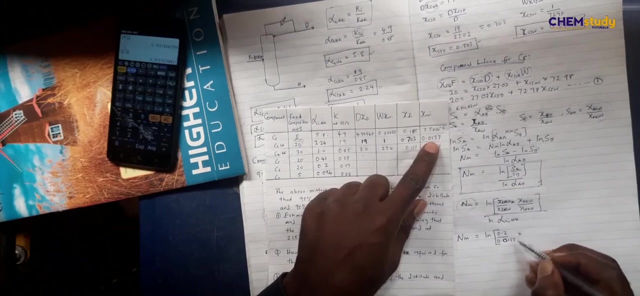 light key in the distillate. x of light key in the distillate. that's 0.2. this is the actual amount, but the fraction is everything divided by 100, because it is 100. so it's 0.2 at the bottoms. the fraction of at the bottoms is 0.13, 0.0137. okay, multiply by heavy key. 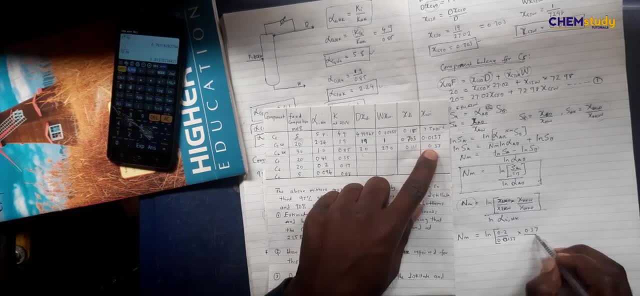 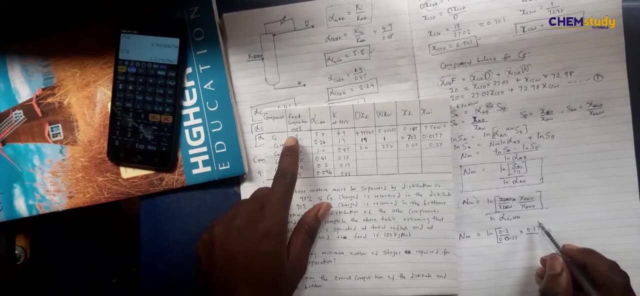 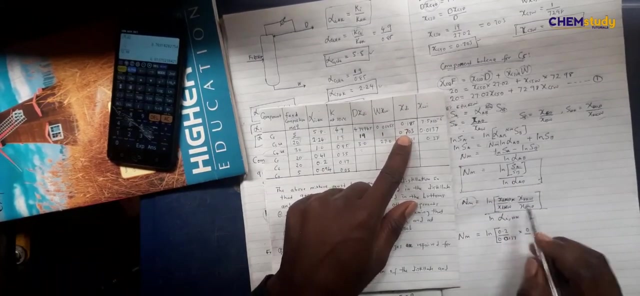 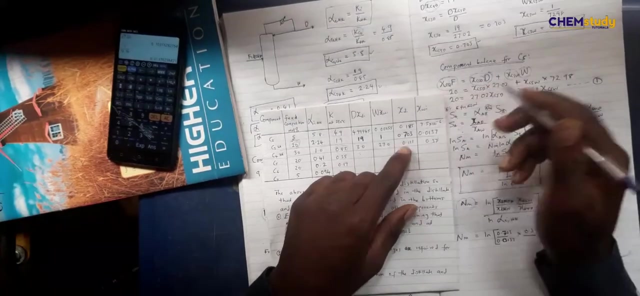 the bottom is 0.37. heavy key at the- sorry, you remember i'm mixing this up. now- is it distillates while looking at not the feed. they said x of light key in the distillate, which is 0.703. okay, there's minor mistakes called cost one max, so let's pay attention to these minor details. 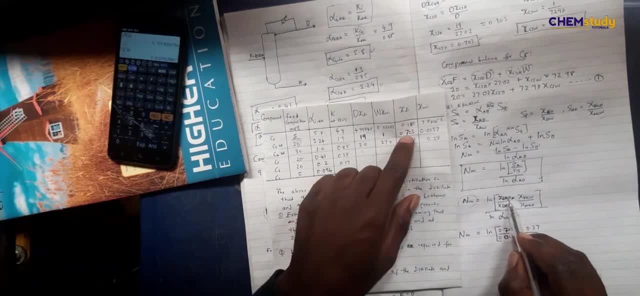 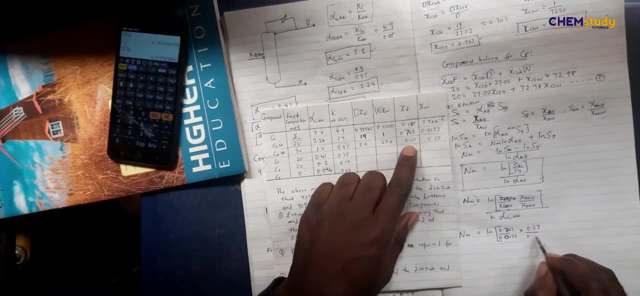 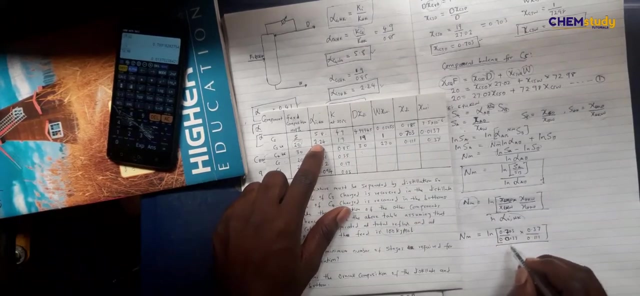 x of light key in the distillate, which is this one: 0.703, this key at the bottoms, is this heavy key at the bottoms, this heavy kid, this latest one tree, one, one, one. the relative volatility light key to heavy key is 2.24. 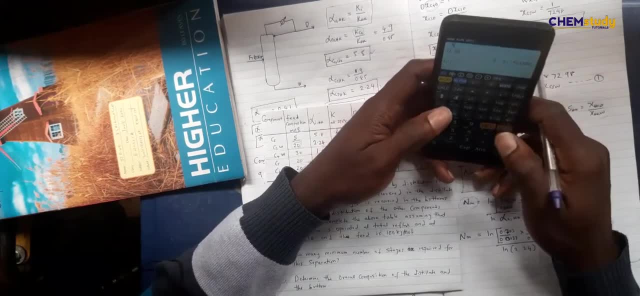 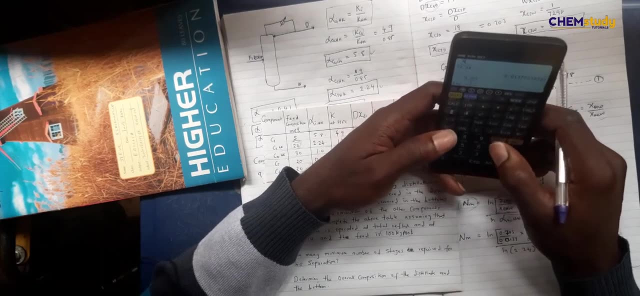 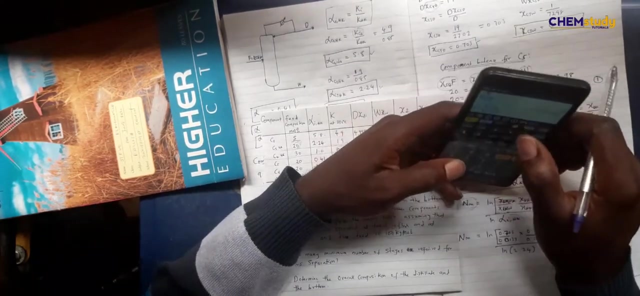 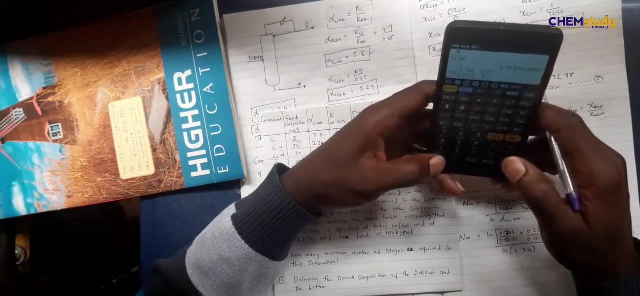 so if we are to do this, we have. we have named 0.703, 0.703, 0.703, 0.703, 0.7, 0.7, 0.前 dilat, 나중에 0.703, 0.0137 times 0.37, so 0.111. 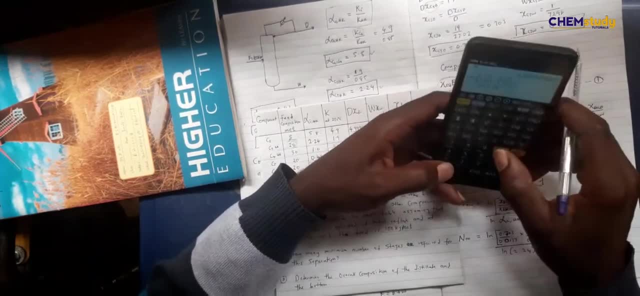 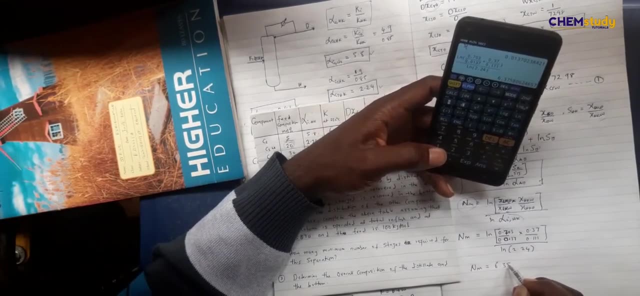 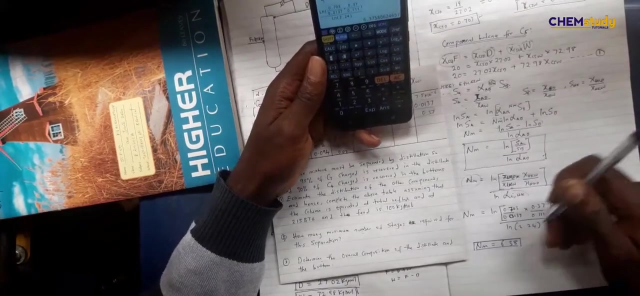 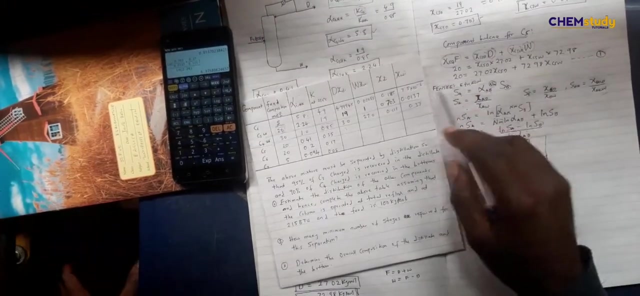 lane 2.24. so our NM is 6.38. so this is our NM, okay, our minimum reflux. this is it here. so now we can go back to this equation, our Fenske's equation for S3. so first from Fenske's equation. 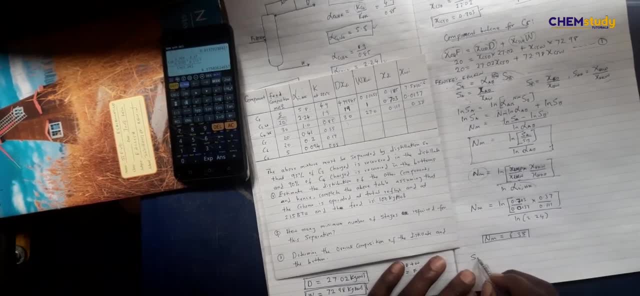 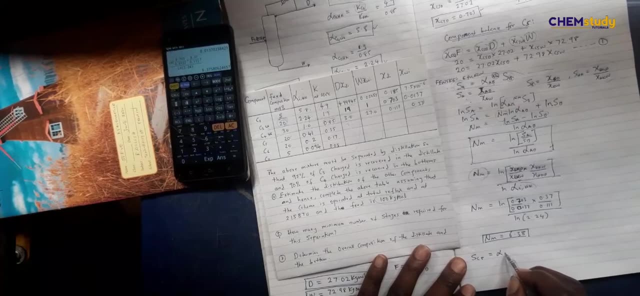 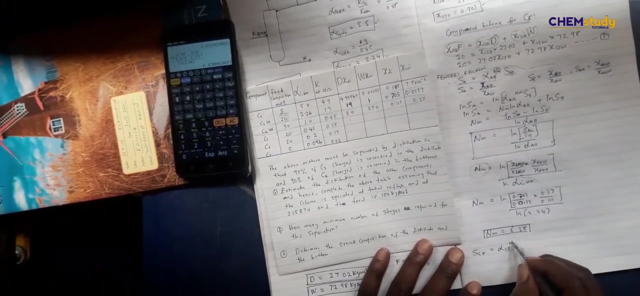 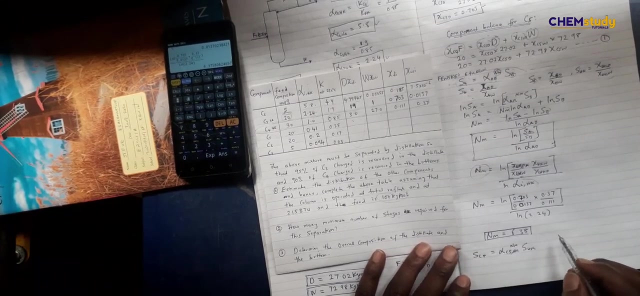 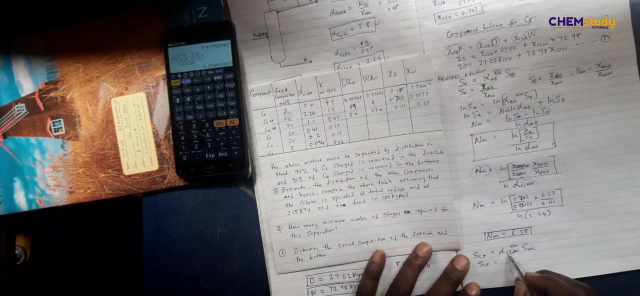 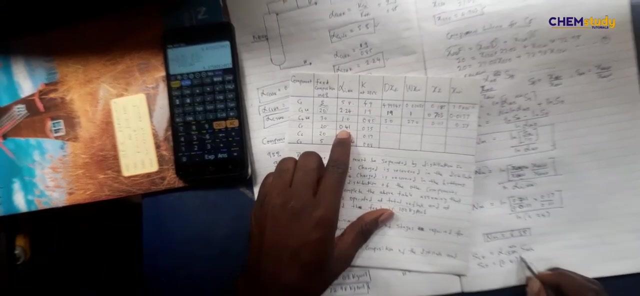 SC5 is equal to alpha C5, NM, C5HK, SHK. okay, so that SC5 becomes 0.011, another SC5 becomes 0.033. that means, what is alpha C5 with respect to hk? there are 0.41. what is NM? 6.38, what is? 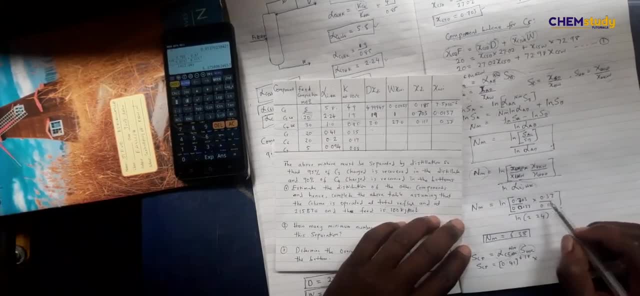 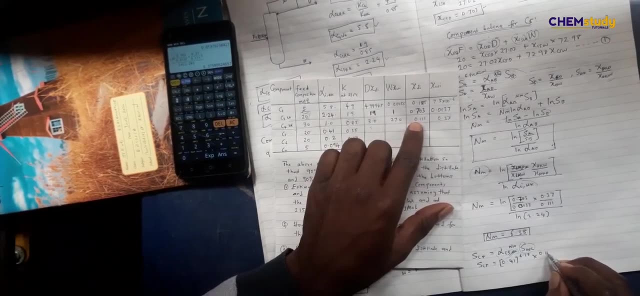 shk. this is sh. shk is heavy complaints in the distillate, which is 0.11, over heavy complaints at the bottom, which is 0.37. okay, so total percentage of- section value of- we will calculate these values in the next. 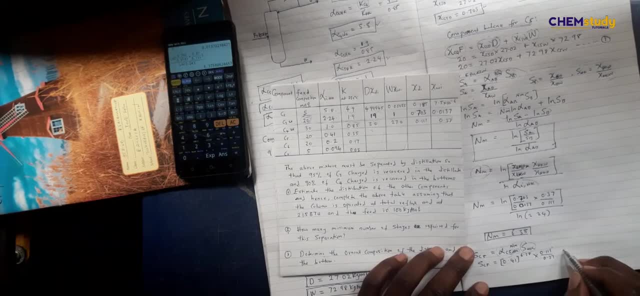 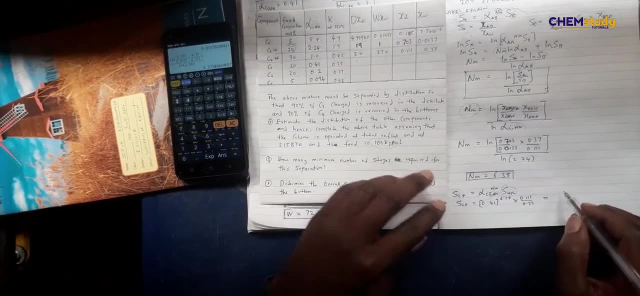 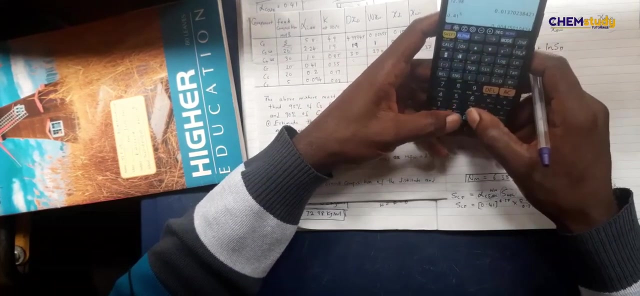 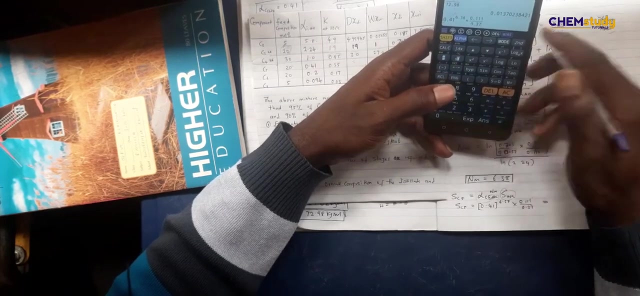 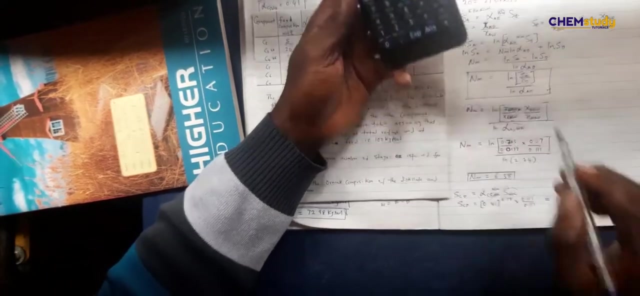 okay, so SC5 becomes 0.41, which is the power of 6.38 times 0.111 divided by 0.37 minus 0.001. you can now remember that SC5 is a split, so the split of C5 now becomes: this is equal. 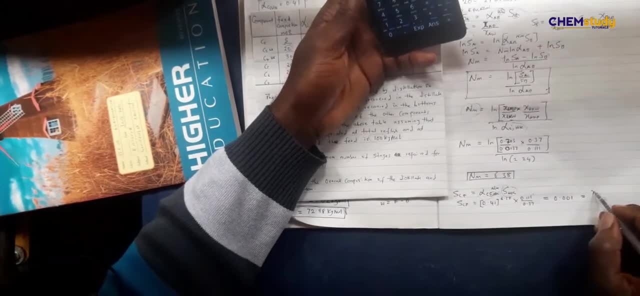 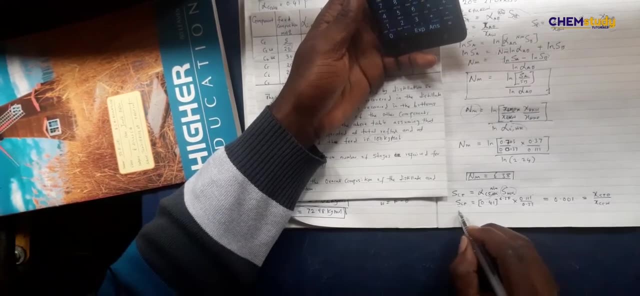 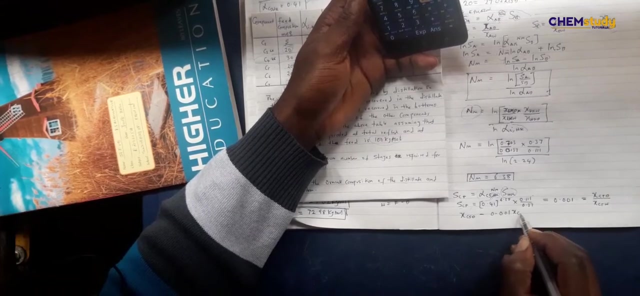 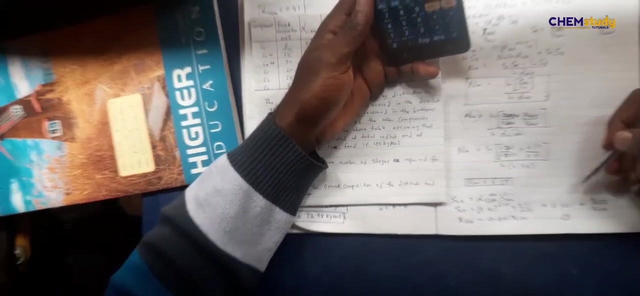 to the split. SC5 is a split that's X of C5 need distillate over XC5 at the bottom. so if we cross, multiply XC5 at the distillate minus 0.01, 0.01 XC5 at the width. this gives us our equation 2, so we solve equation 1 and 2 simultaneously. 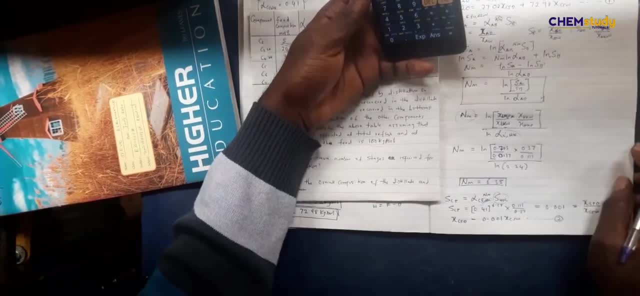 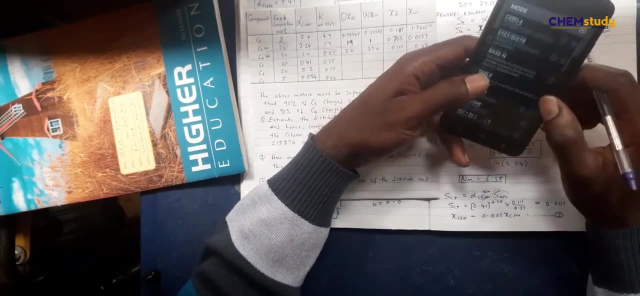 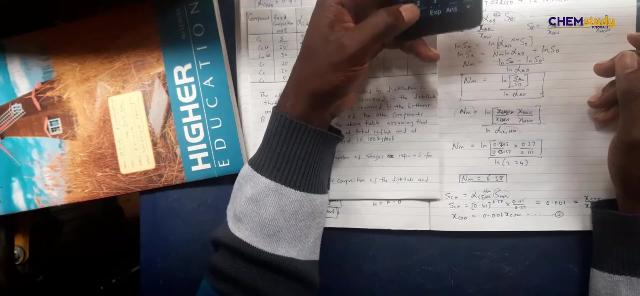 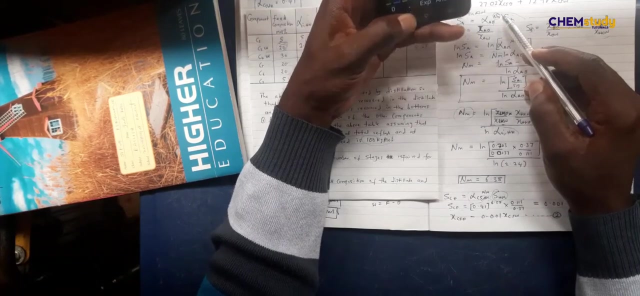 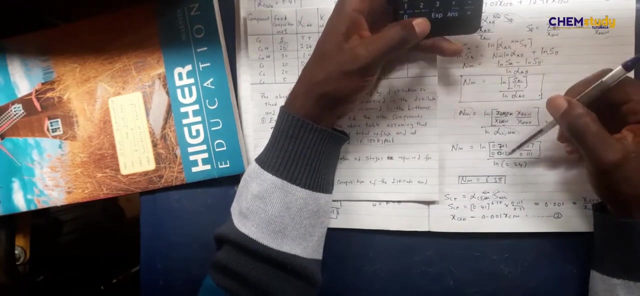 let me show you this working. okay, so you solve equation 1 and 2 simultaneously. now, if I solve them simultaneously, I just want to use my calculator: 27.02, 72.98, 21 minus 0.001, so equal to 0, remember. 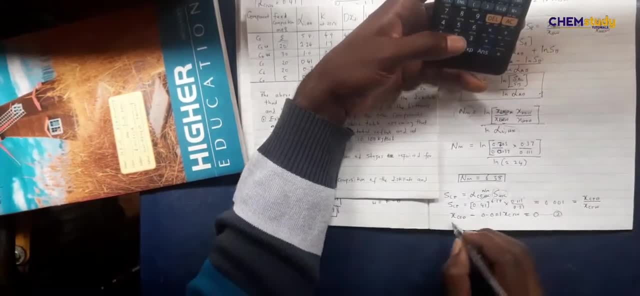 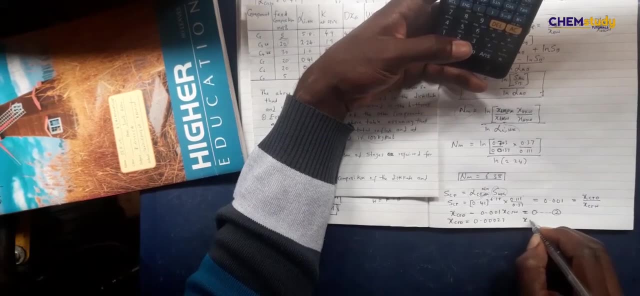 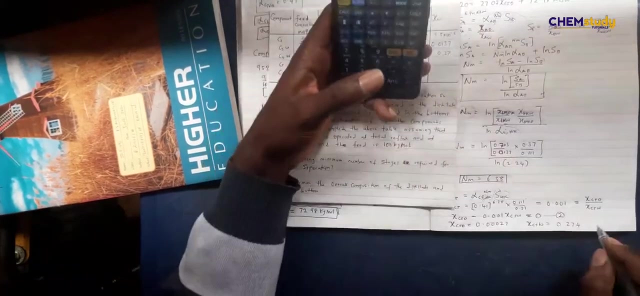 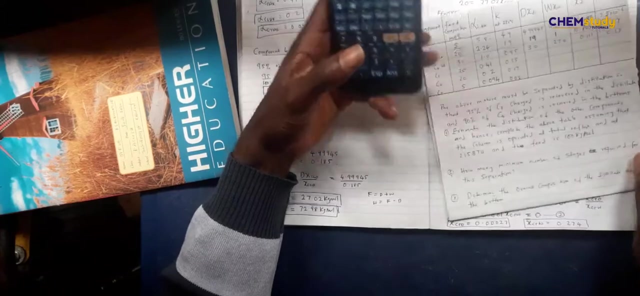 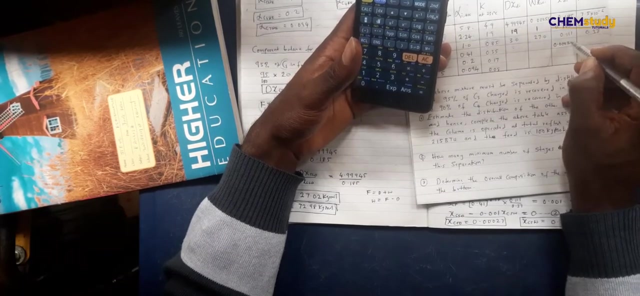 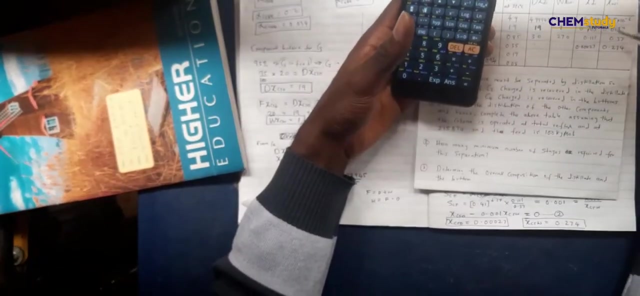 so our X of C5 in the distillate becomes 0.00027 and X of C5 at the bottoms becomes 0.274. that's how we find this C5 needs distillate 0.0027. so you see, these results even makes sense in that value of XC5. no, C5 is heavier than heavity. such value or word of Java does not have an half litre. half litre C5 is heavier than a half litre C5. so in that form, in that 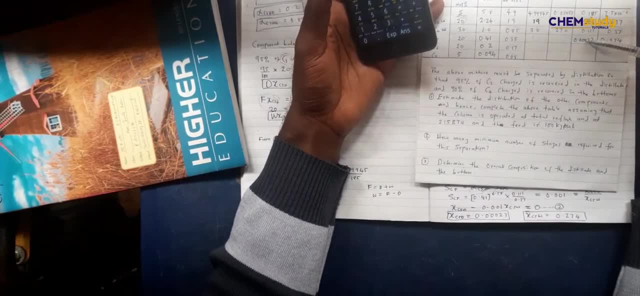 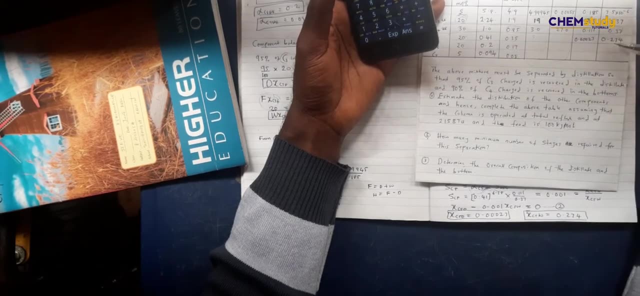 xc5. you know c5 is heavier and heavy, so the value of xc5, xc5 also, Tesla وا- is going to change length of the circle. so the value in the distillate begins to drop drastically, while the value drops drastically, while the value of c type in the waist is still gaining weight. so that's how we work. 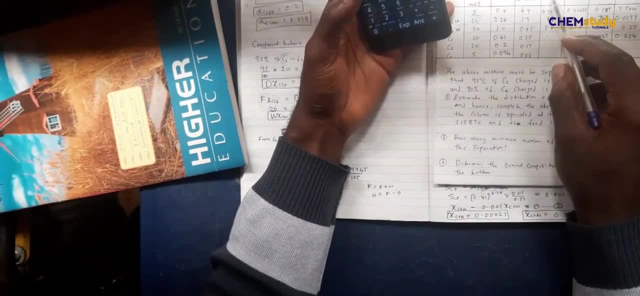 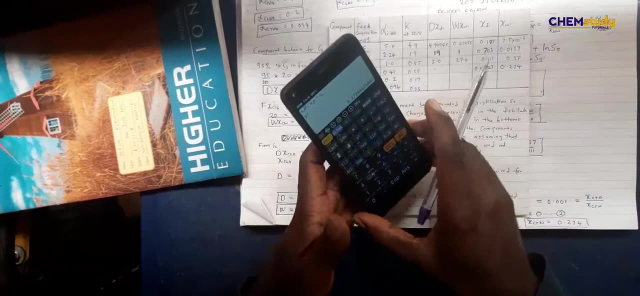 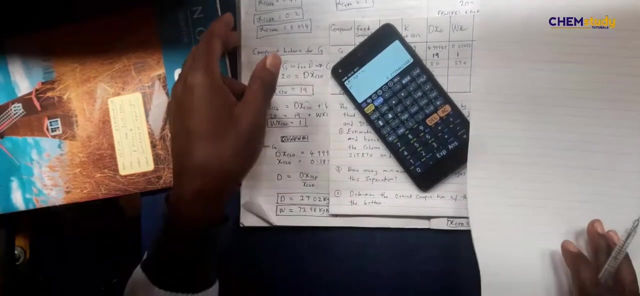 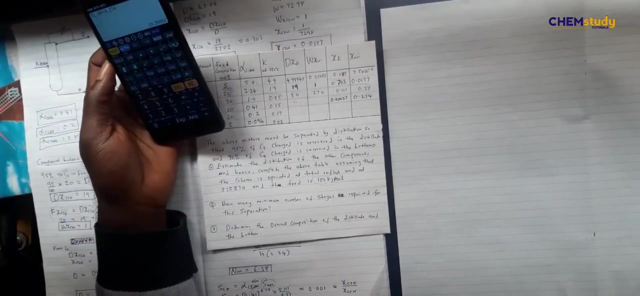 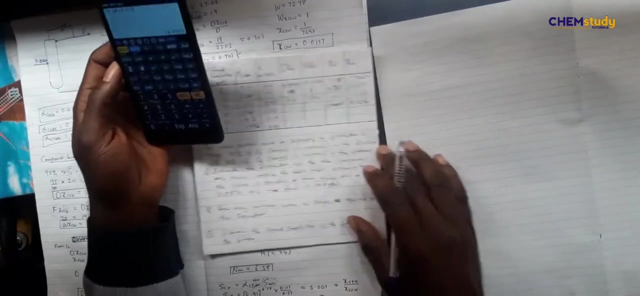 then the next thing is to find the d and w. so remember to find the d. let me bring another paper so we just continue. so to find the d, okay, just be sure everything is set. so to find the d. simply, you know we have, we know the value for d. 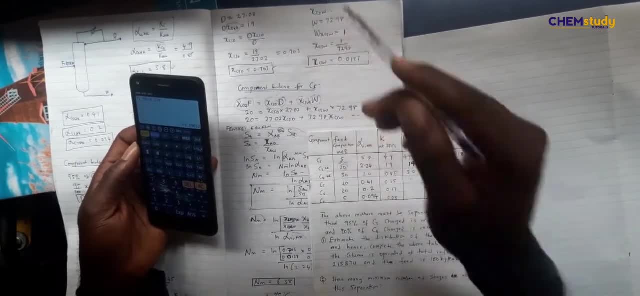 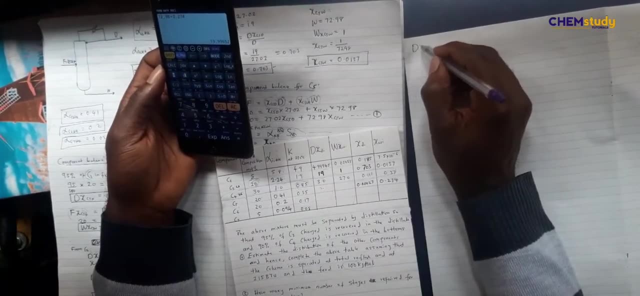 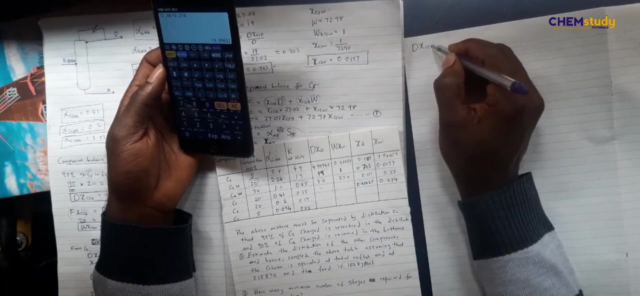 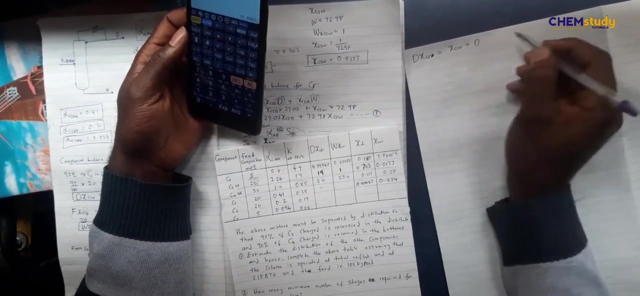 as 27.02 and we know xdi and xw ui. so d x c5 in the distillate becomes x of c5 in a distillate times d. what is x of c5 in the distillate? that's what we found. 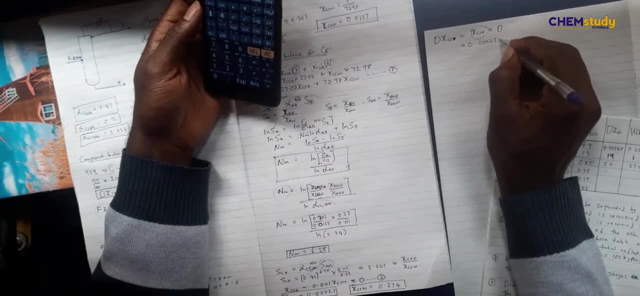 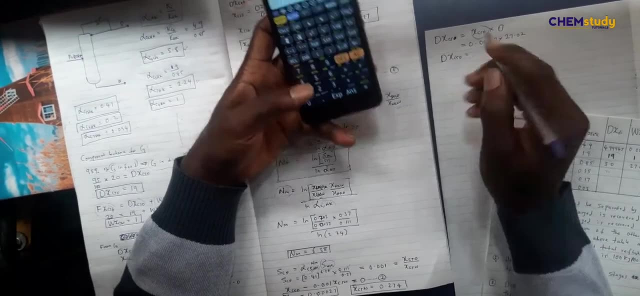 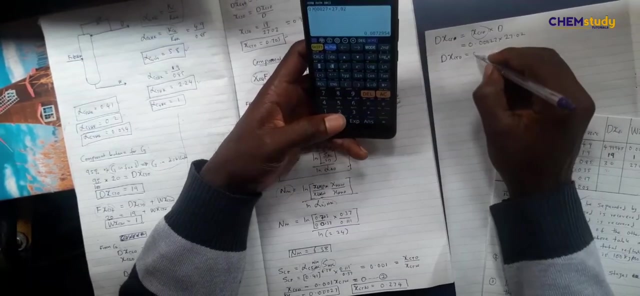 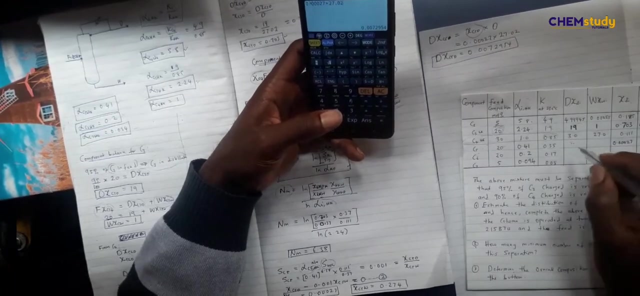 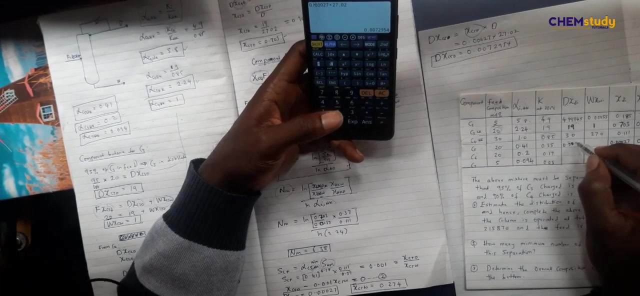 as zero point zero, zero zero, two, seven times what's the distillate, 27.02. so if you times this d x of c5 in, the distillate becomes 0.007295. so you go to your table 0.00 seven three okay. 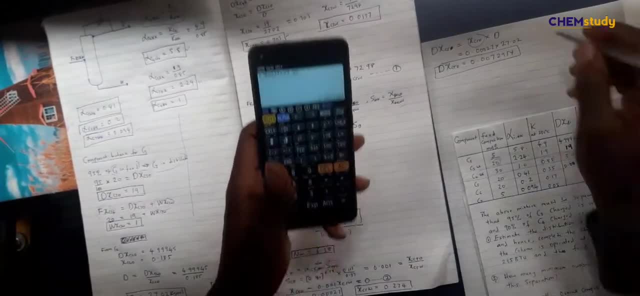 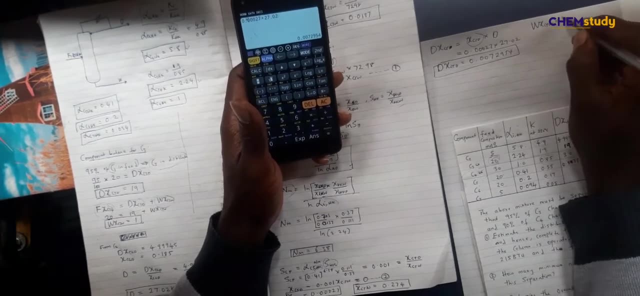 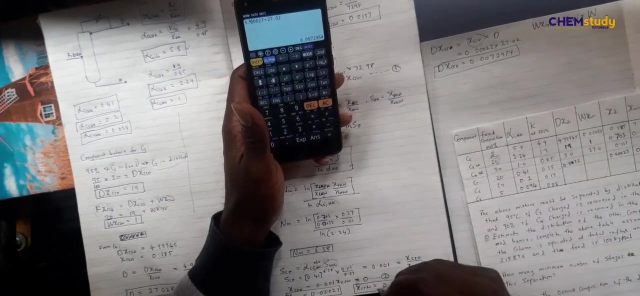 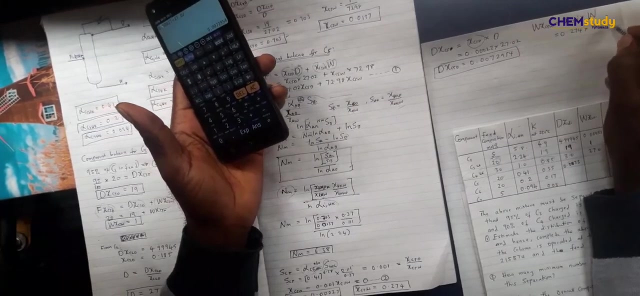 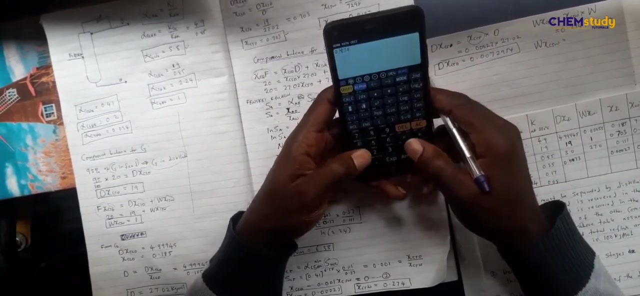 so, then, to find the value of w, w um xc5w, simply the same thing: xc5w times w, so xc5w. we just found it to be 0.274, and w is 72.98 to w, xc5w, because 0.274 times 72.98 that's 19.997. 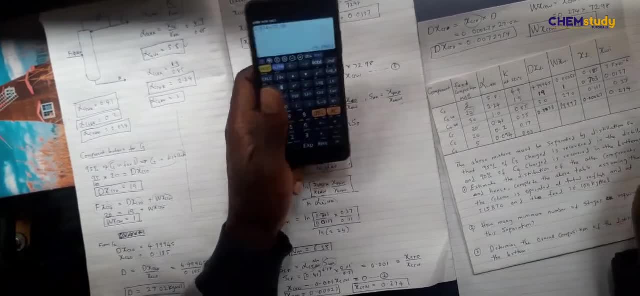 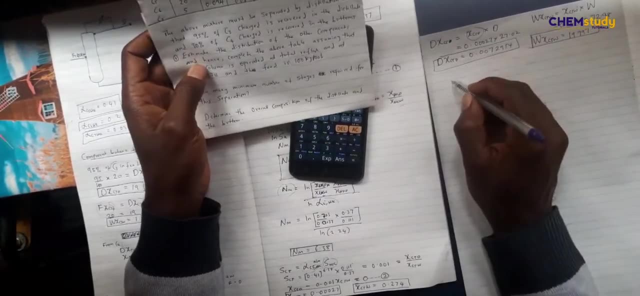 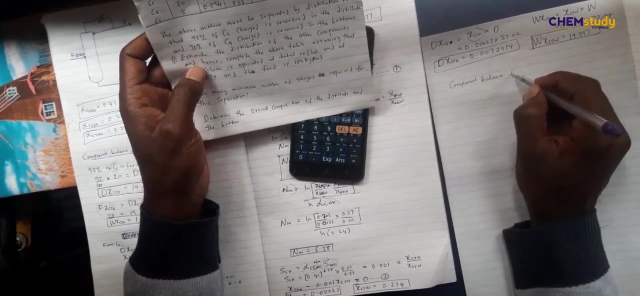 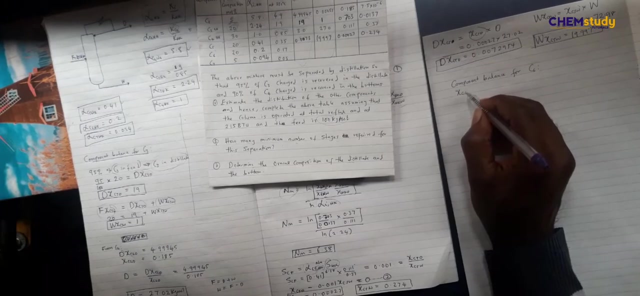 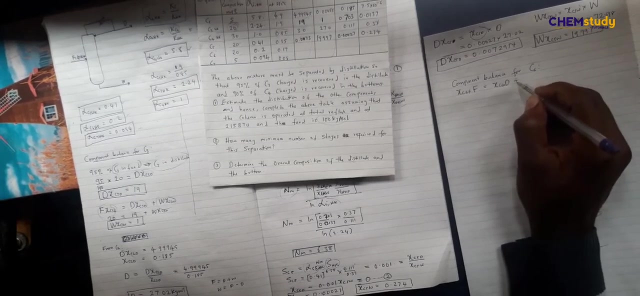 so you fill it in your table: 19.997. so, um, we have two columns left, so component balance four. so continuing on. okay, so this is what we have here, so we can simply do the same thing we just did. so i'm going to change this, we're going to 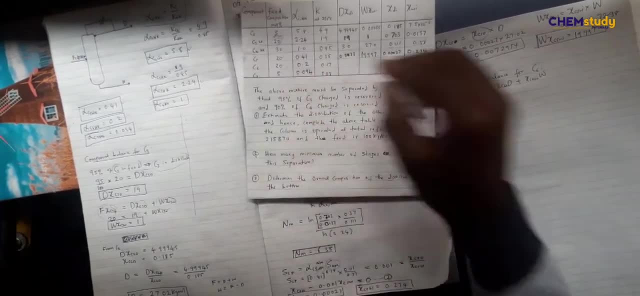 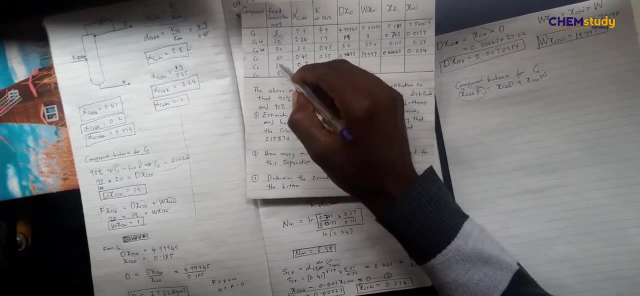 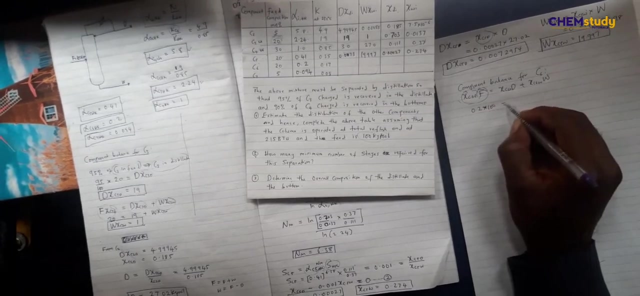 change it to a new column. so xc6, so fc6. in the feed times the field is equal to xc6 in this little. this is like plus xc6 at the bottoms times. the bottoms, the feed is 100, so either it gives you 20. x in the distillate? we do not know it. 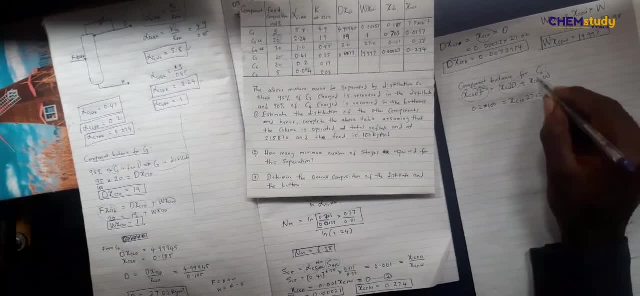 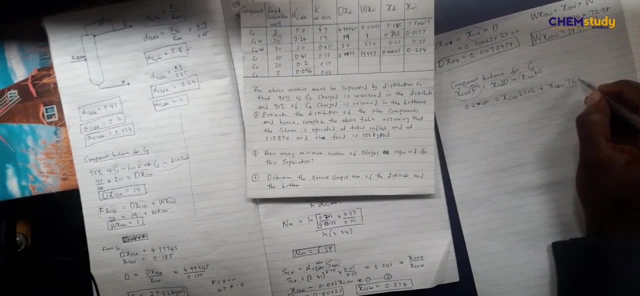 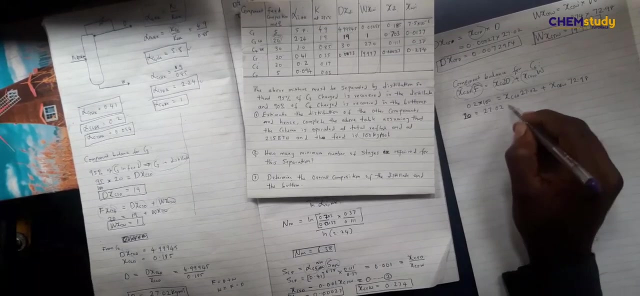 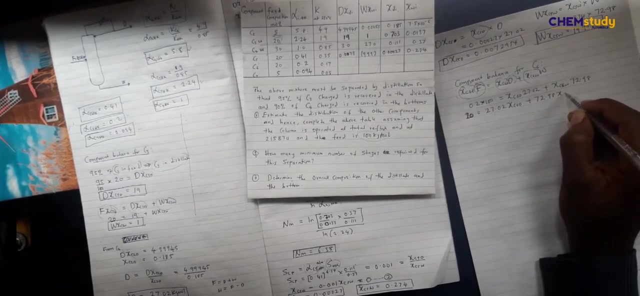 the distillate is 27.02. we do not know this where the waste is 72.90. so we have one. we have 20, equal to 27.02 xc6d plus 72.98 xc6w. so this is equation one. so final equation two: we do not need to find nm. 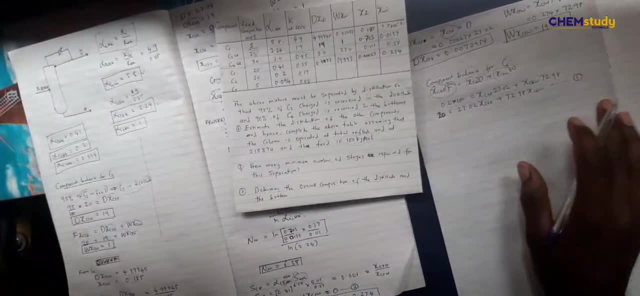 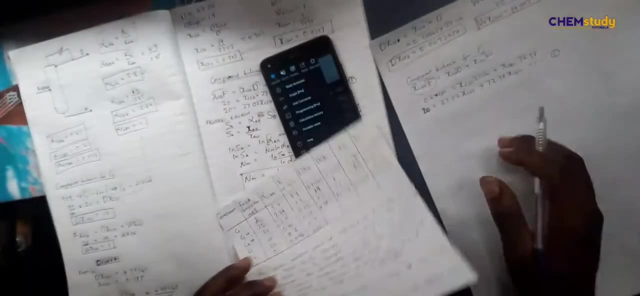 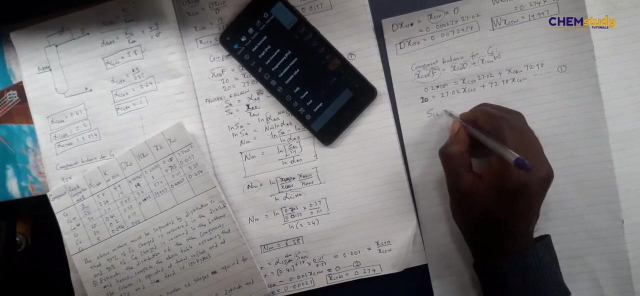 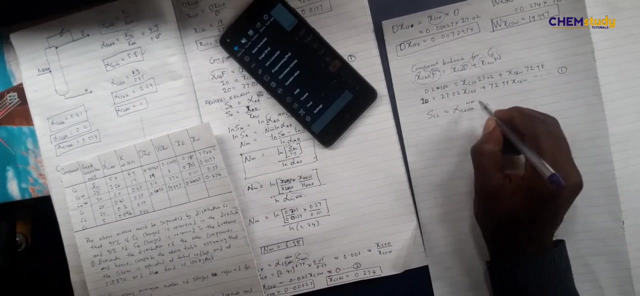 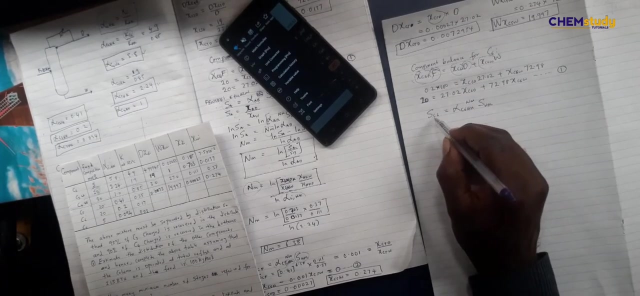 from the scratch anymore, because we already know the value for nm. so what we do is simple: from from this stage. from this stage, sc6 becomes what is the relative latitude of c6? hk and relative latitude, i'm sorry, split of hk, so split of c6. 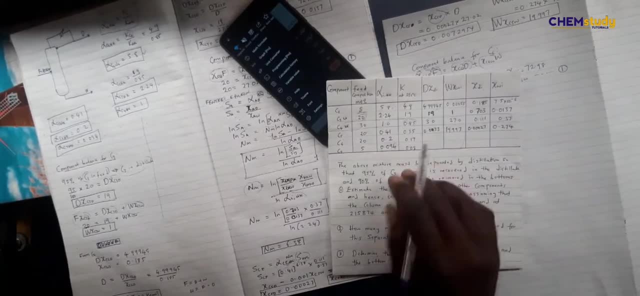 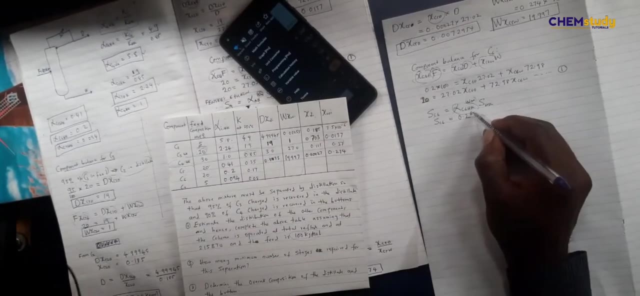 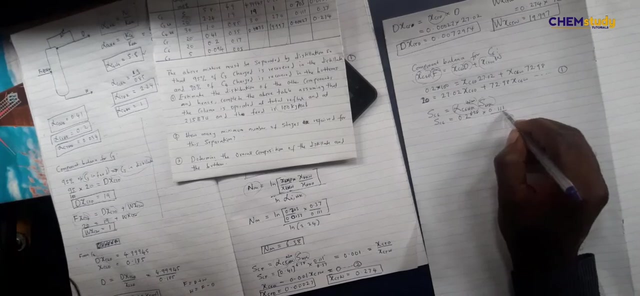 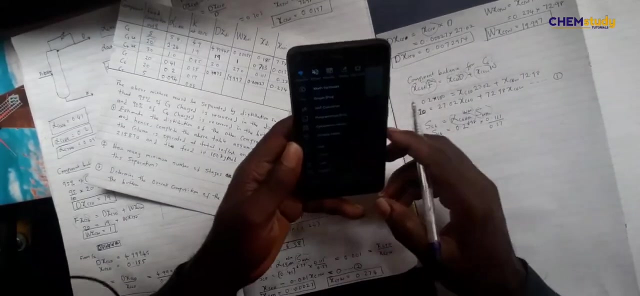 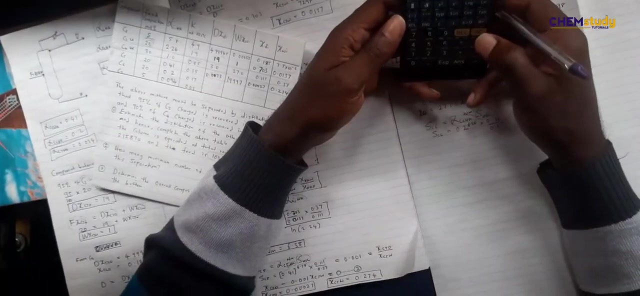 becomes what's the relative latitude of c6? hk 0.2? what is nm 6.38 shk is 0.111 divided by 0.37. okay, so this becomes 0.2. we use the power of 6.38. 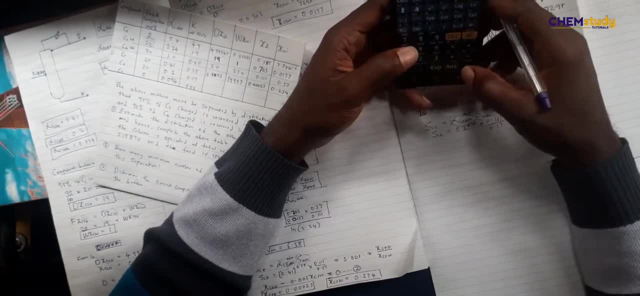 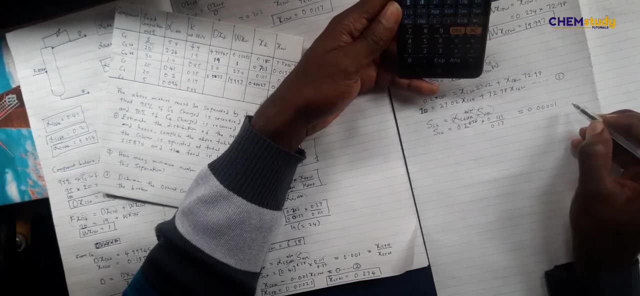 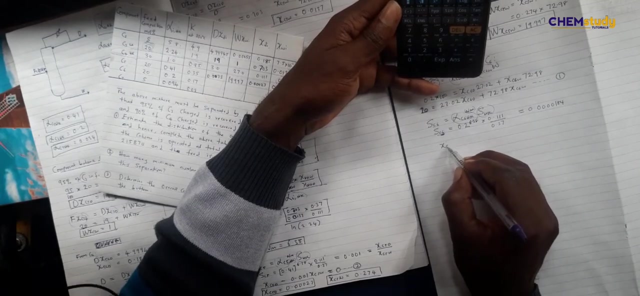 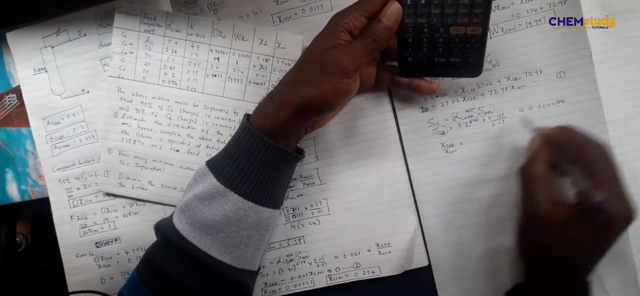 times 0.111, 0.37, so xc6 becomes 0.0001, 0.04 and we are. split simply means c6 in the distillate over the fraction of c6 at the bottom. that's the meaning of this and it's equal. 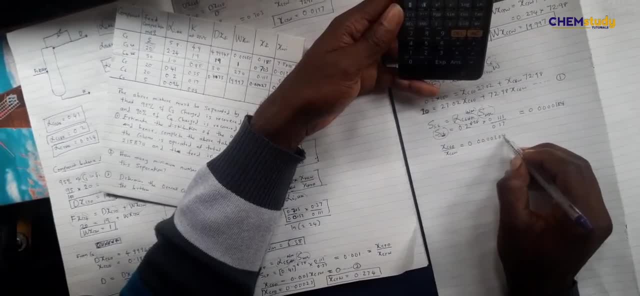 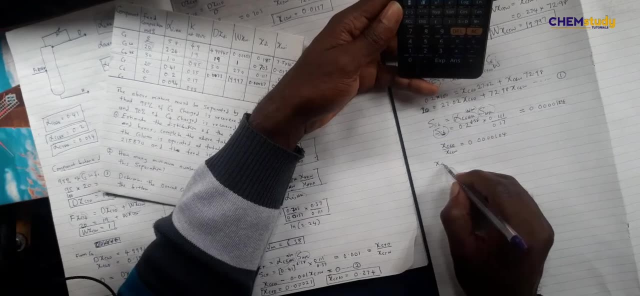 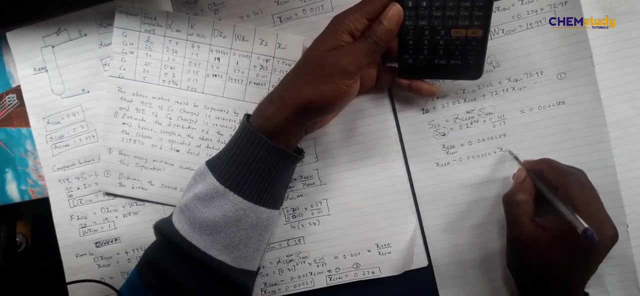 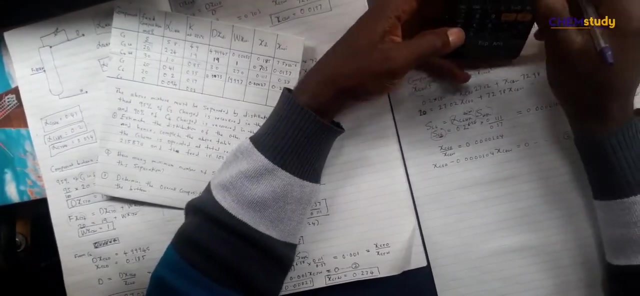 to zero point zero, zero, zero, zero, one zero four. so if we cross, multiply and bring everything to one side, x c6 in the distillate minus zero point zero, zero, zero, zero, one, zero four. x c6 at the bottom equal to zero. this is equation two, solving both of them simultaneously. 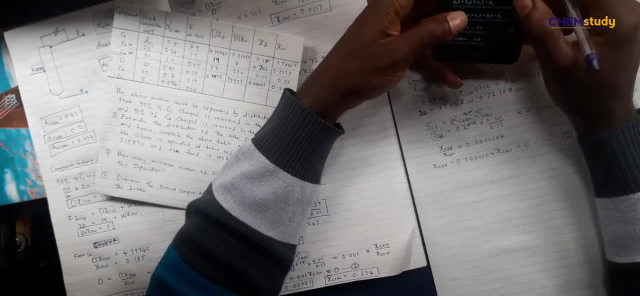 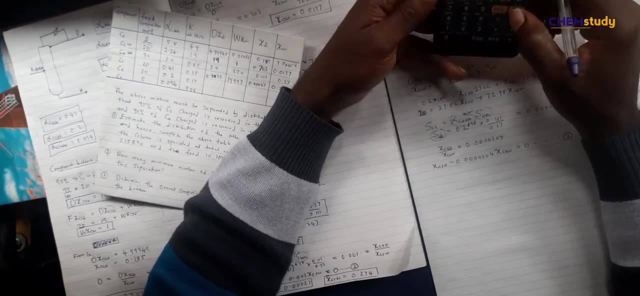 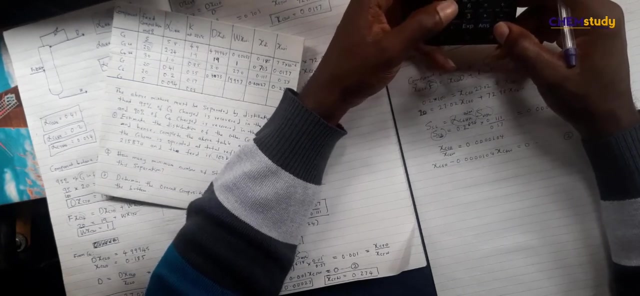 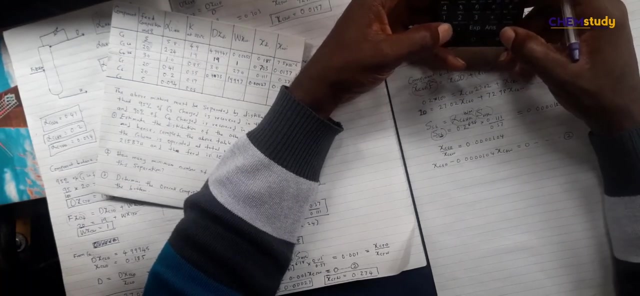 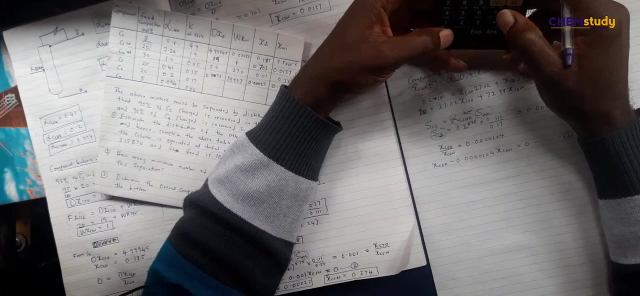 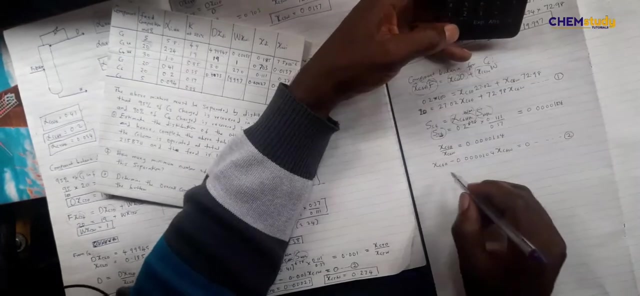 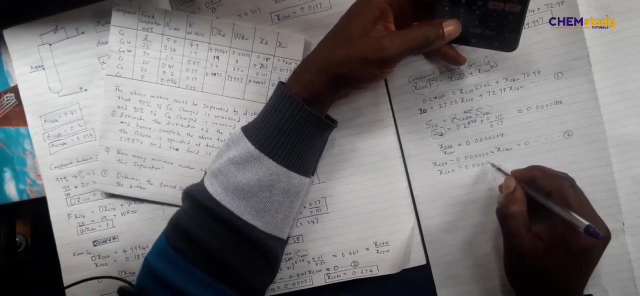 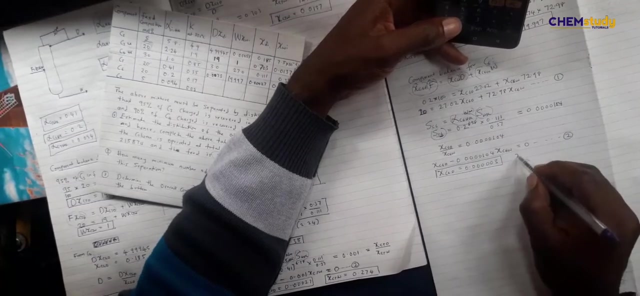 we have um, okay, we have a igesin, We have 27.02,, 72.98,, 20, then we have 1, minus 0.00000, 104.. So XC6D becomes 0.000003, and XC6W becomes 0.274.. 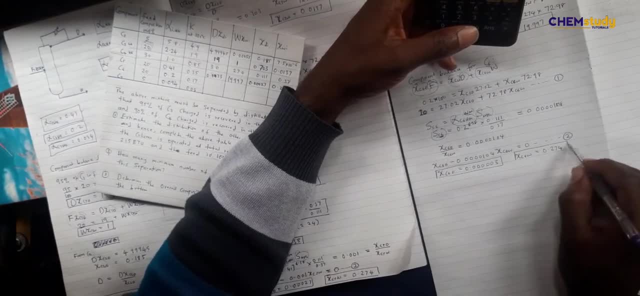 So we have 27.02,, 72.98,, 20,, then we have 1, minus 0.00000, 104.. So XC6D becomes 0.000003, and XC6W becomes 0.274.. 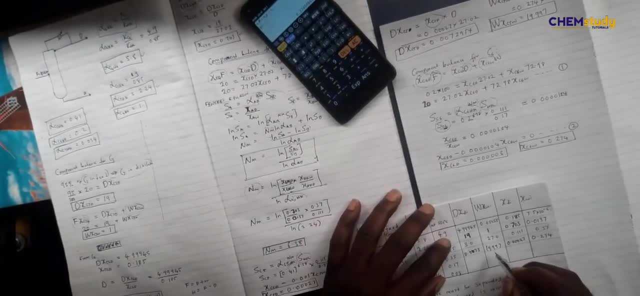 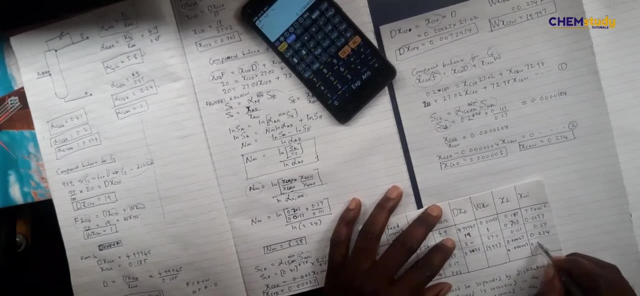 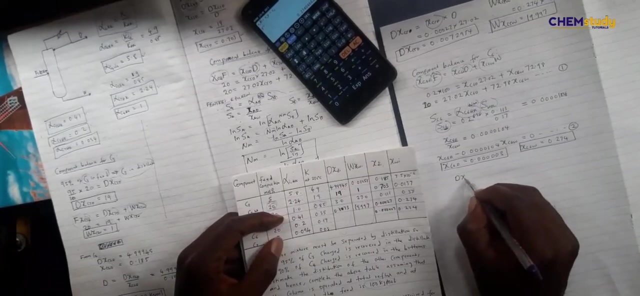 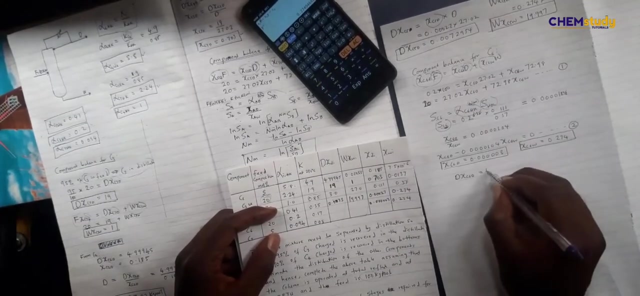 So these are our answers. So 0.000003 answers 0.274.. So, like we did before, to get the XC6D, simply the value for D, simply D times XC6D, D is 4.. 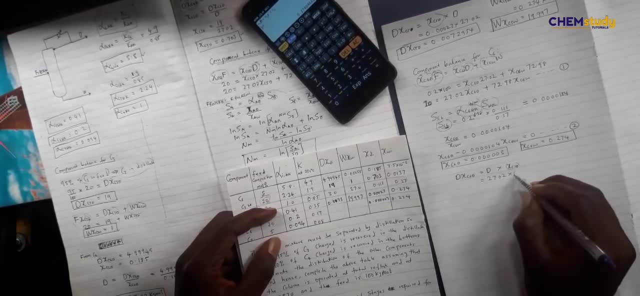 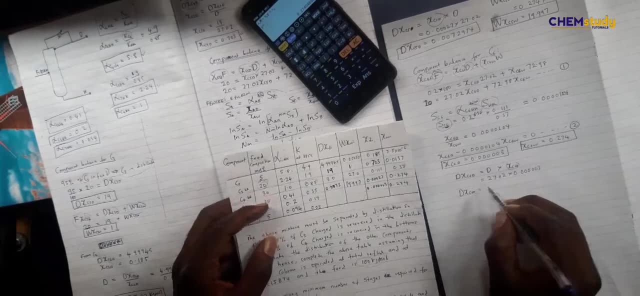 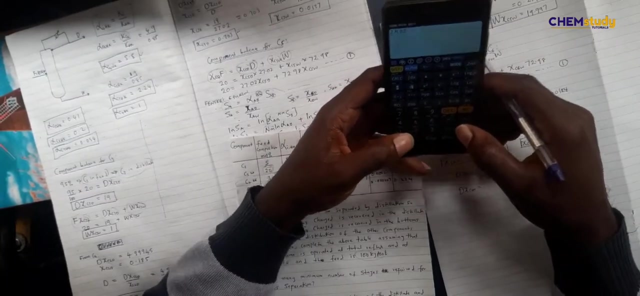 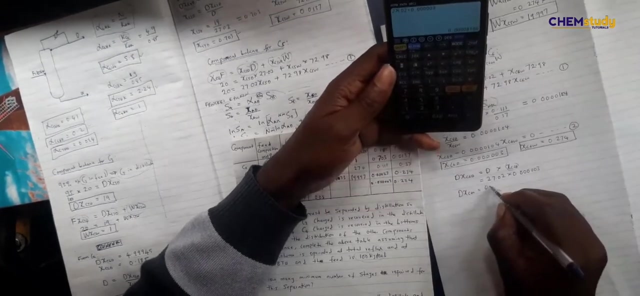 D is 27.02.. This is what we just found. So D XC6D becomes 27.02 times 0.1034.. So it becomes 0.0000.. 0. 0. 0.. 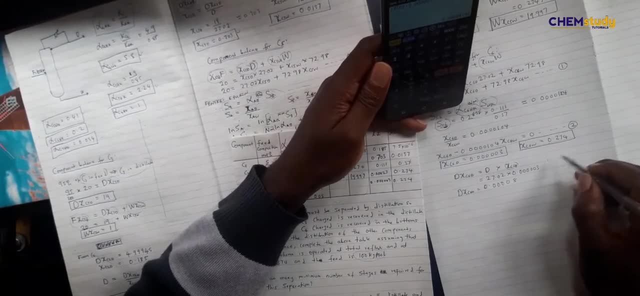 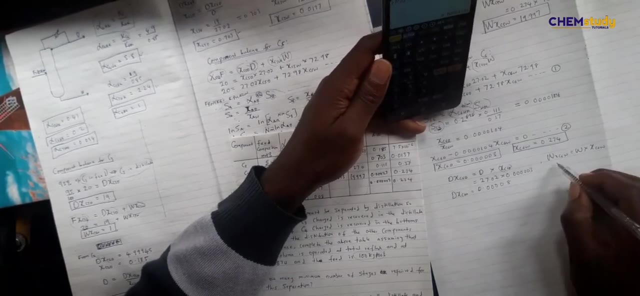 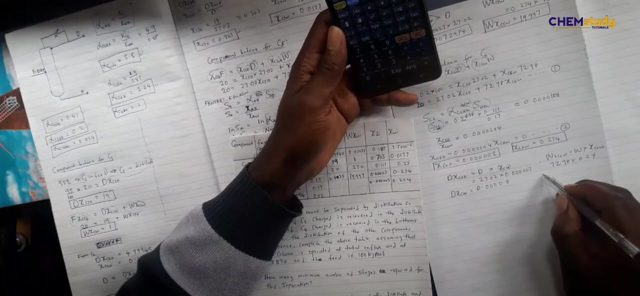 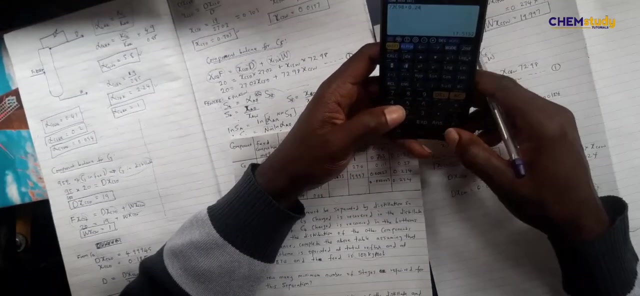 0.. 0.. 0.. 0.. While W XC6W becomes W times XC6W, So that's 72.98 times 0.24.. So W XC6W becomes 17.5152..